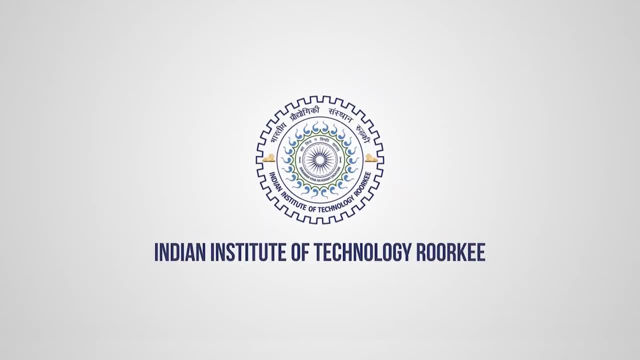 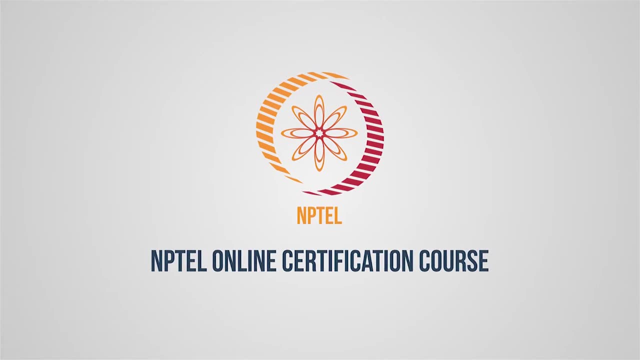 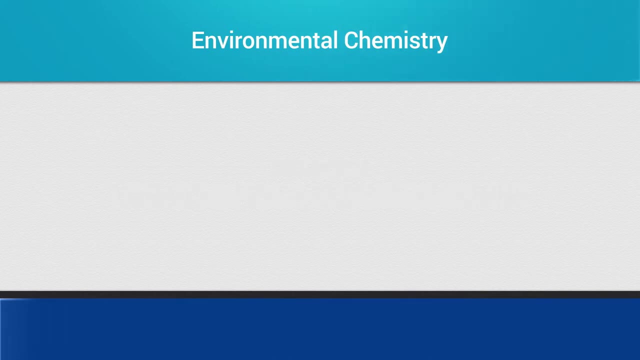 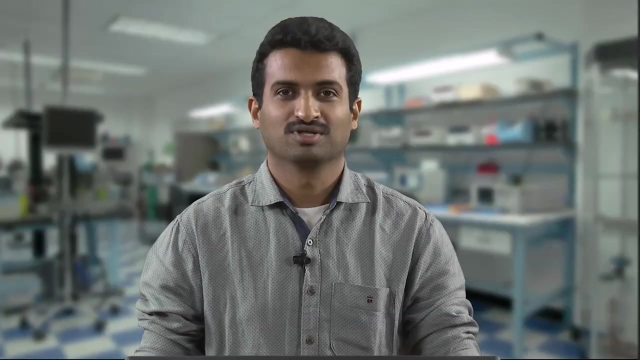 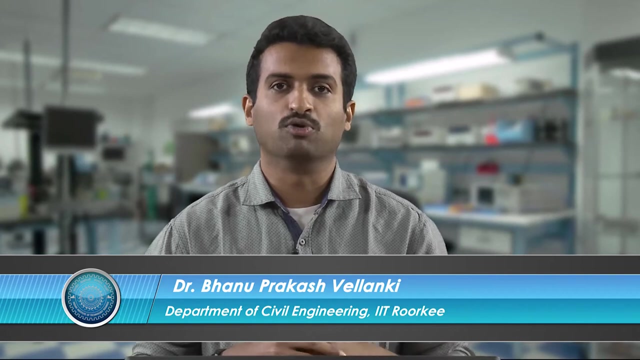 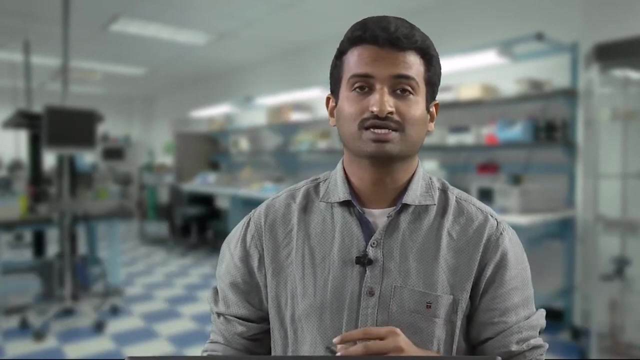 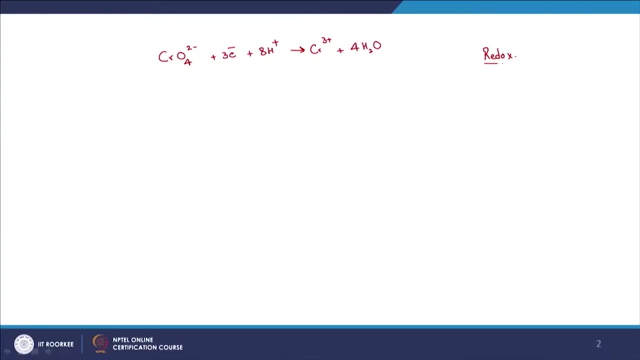 Hello everyone, Welcome back to our latest lecture session. Let us have our customary review for a few minutes about what we have been up to in the last couple of sessions and then continue with where we left off. We were looking at reaction feasibility or with respect to equilibrium, We were discussing redox reactions and we looked at different 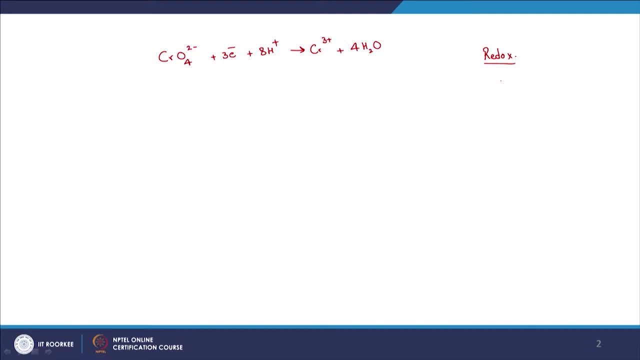 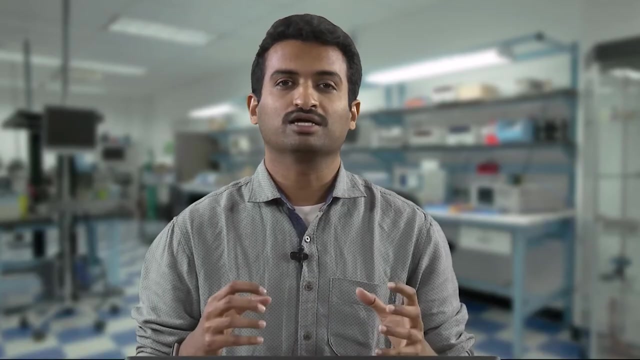 terms- electron acceptors, donors- and then we moved on to discussing kinetics. We were done with that and we started discussing about equilibrium, and we are just going to quickly recap what we have been discussing with respect to equilibrium. As we mentioned or discussed most of these redox processes, though they are feasible, 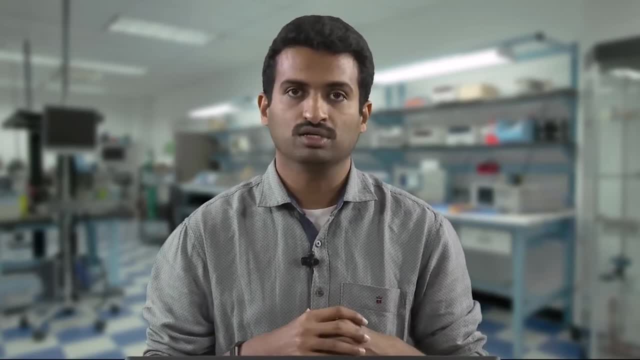 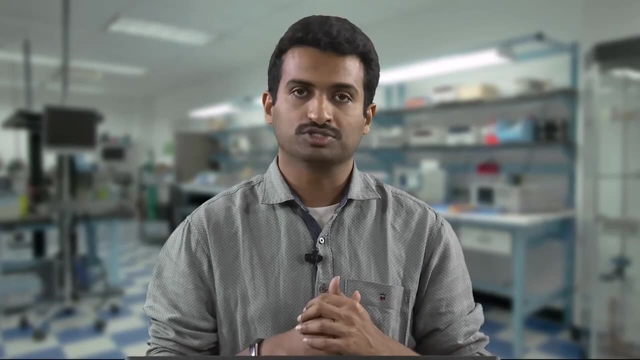 they will not go through because of the kinetics being way too slow. In general, what is the norm? Redox, disequilibrium is the norm. That is something that we have understood from our last couple of sessions, But looking at equilibrium will help us in understanding. is the reaction feasible or 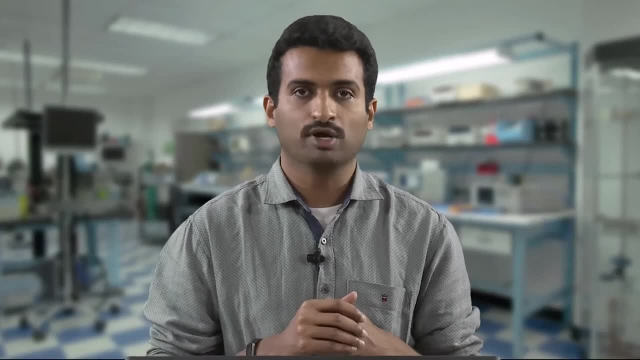 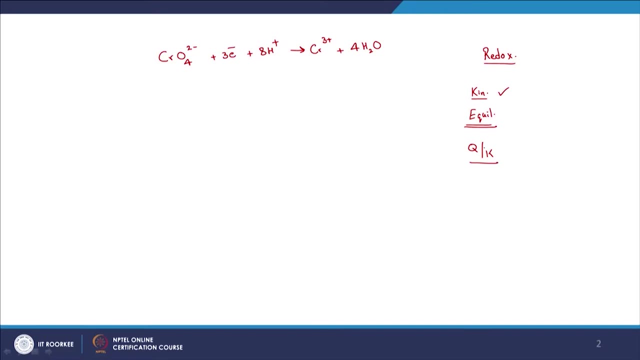 not feasible. In that context, we looked at two approaches and one of the approaches was looking at Q by K. How did we get here For one half reaction? we can calculate K1 or we not calculate, pardon me. we can obtain the relevant K1, equilibrium coefficient. 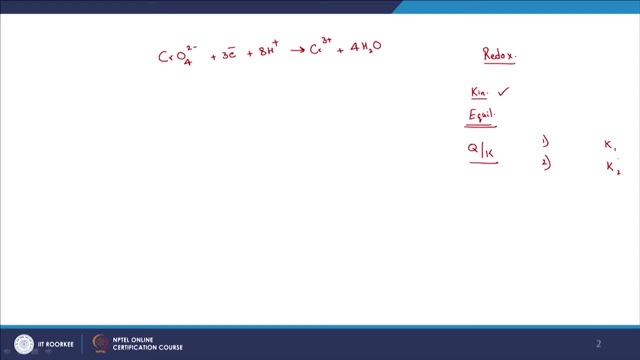 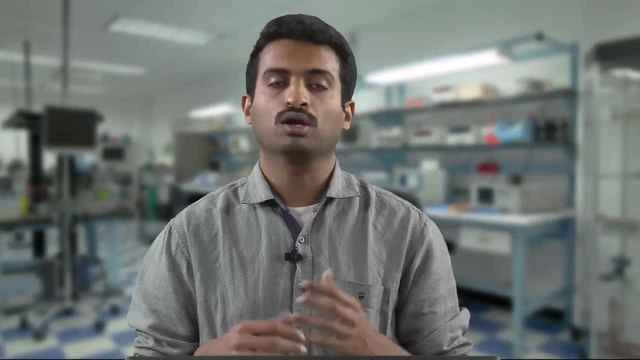 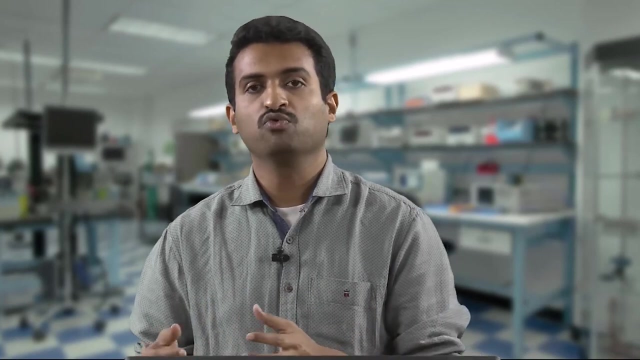 For the second half reaction, get the relevant equilibrium coefficient And then you are going to sum up 1 and 2 after modifying either reaction 1 or reaction 2, so that you will equate the number of electrons being transferred. and then we saw how we can. 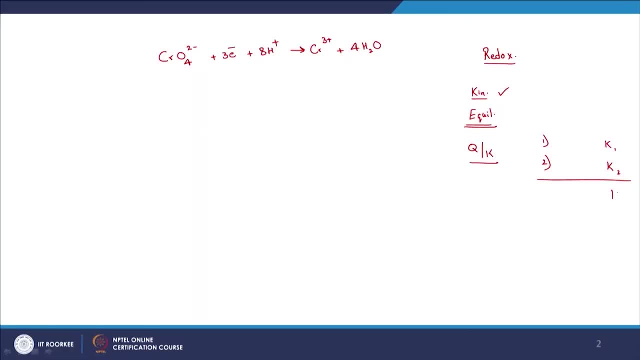 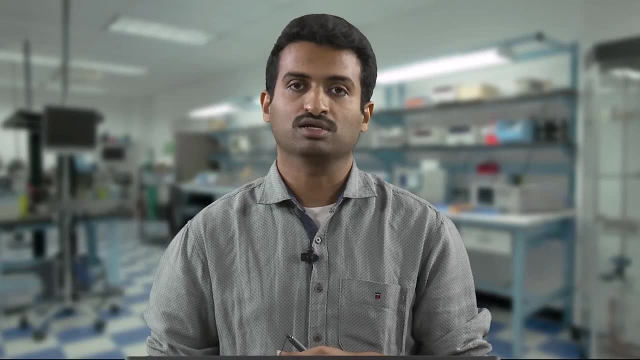 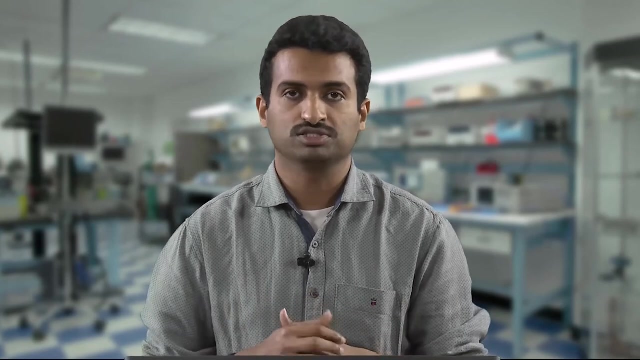 come up with our particular K for the overall reaction. For the overall reaction, we looked at how to calculate that particular equilibrium coefficient And the key is that we need to situate that the number of electrons being transferred would be the same And both this reduction and oxidation process are the half reactions. 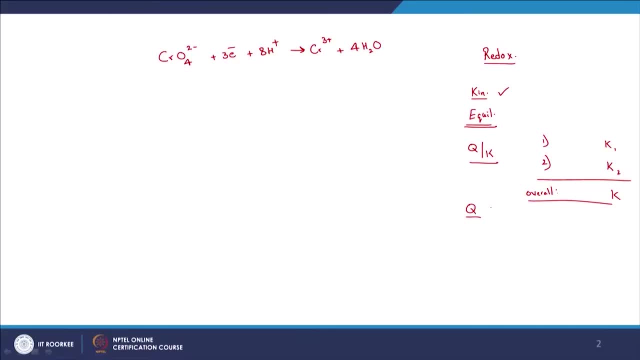 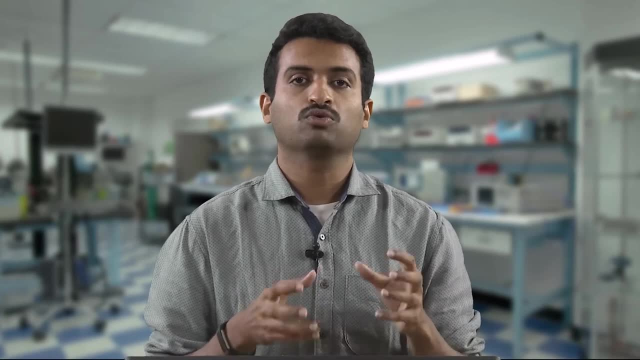 We did that, and then you can calculate Q based on the relevant concentrations that you have in your particular system. Q will tell you an idea about what is the present scenario. K will give you an obvious idea about what is going to be the system or how is it going. 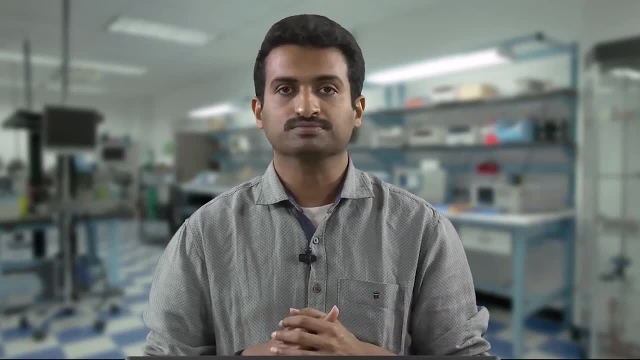 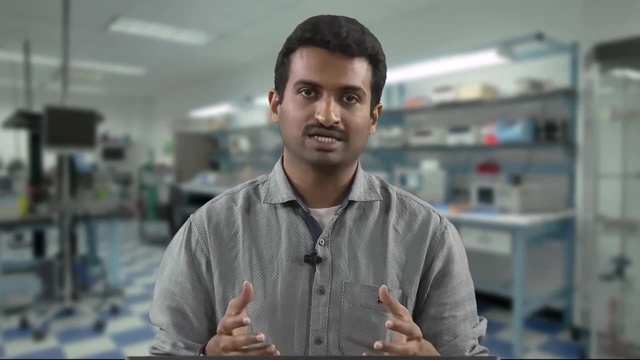 to be at equilibrium. When you look at Q by K, and obviously if Q by K is less than 1, it means that the reaction is feasible. Equal to K, it means it is at equilibrium, and greater than K, it is not feasible. 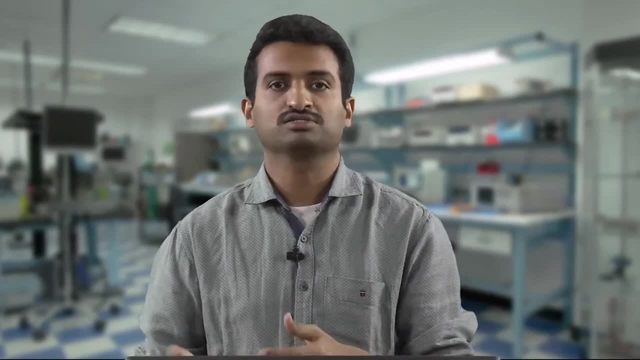 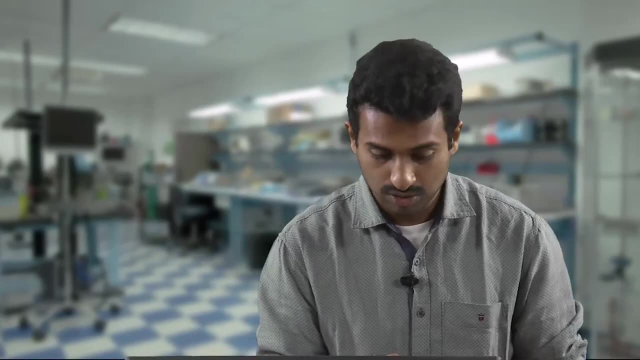 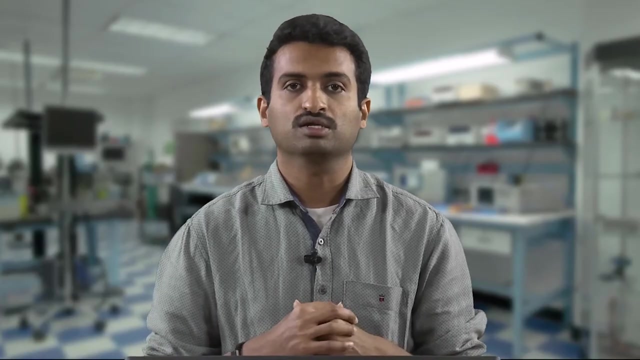 That is something that we looked at in some of the previous classes and that is something that we looked at from the point of view of the redox process. And then we started looking at new approach or a different approach, something that we have not looked at yet: the reduction potential or the PE. 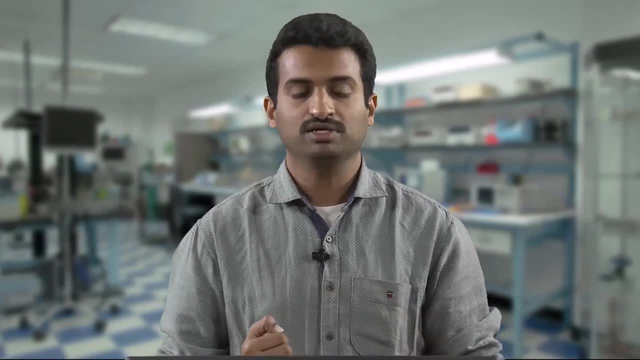 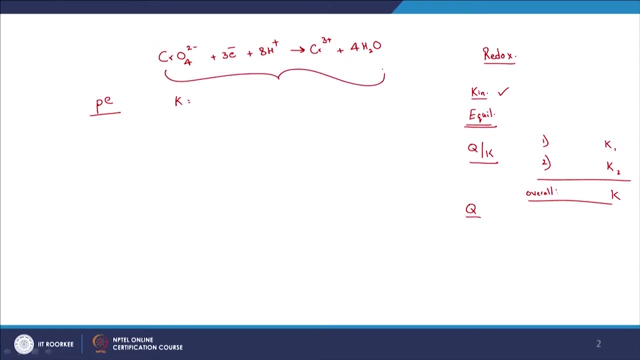 In this context, we first looked at how to get at that PE. how did we get that? we wrote down the equilibrium coefficient for a particular equation and this is the particular example I believe we looked at. We looked at the particular equilibrium coefficient, stoichiometry of the products, so their coefficients. 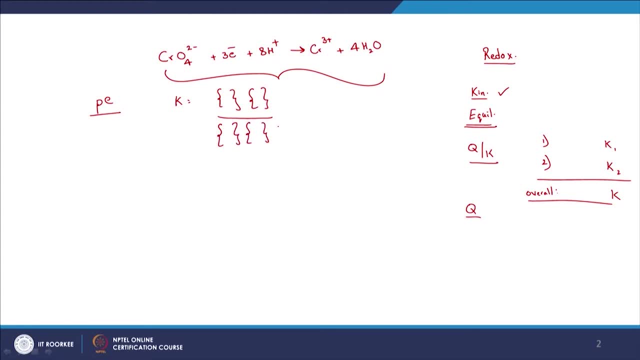 biased activities of the relevant- what is it now? the relevant reactants. we got that done and then we plugged it in, transformed the equation such that more or less, we end up with PE equal to Pe0-1 by m. Okay, 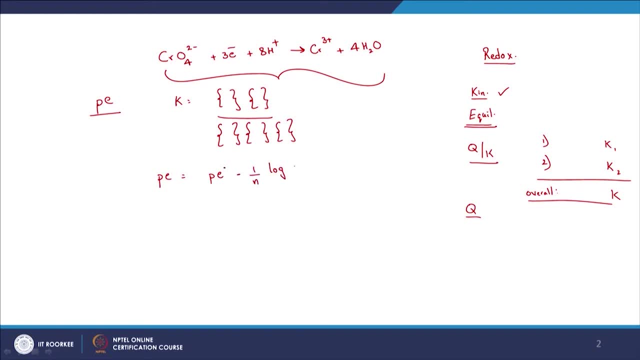 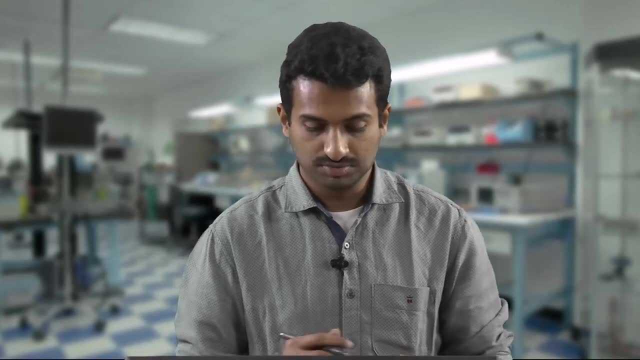 Okay, Okay, So it is 1 by n log, Q, dash. So let us try to refresh what it is that we need to understand with respect to each of these terms here. So PE is your reduction potential, which is what we are going to consider with respect. 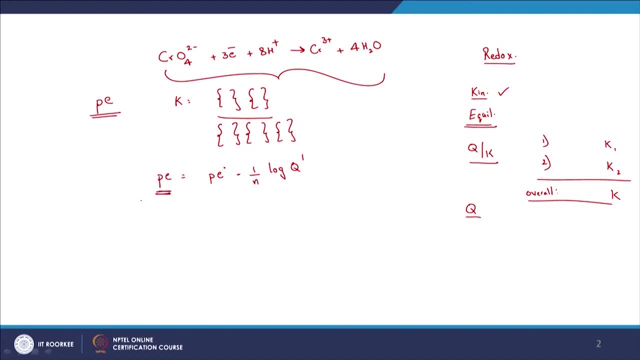 to determining our redox reactions, feasibility And Pe0. if you look at how we derived that, it was equal to 1 by n log K. So it gives you an idea about the system at equilibrium. So Q dash is nothing but Q multiplied by the electrons rise to the stoichiometry of 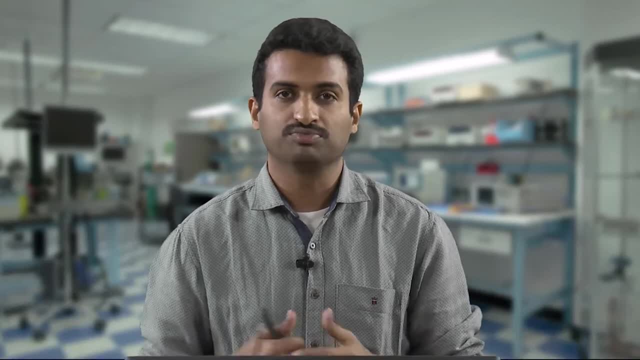 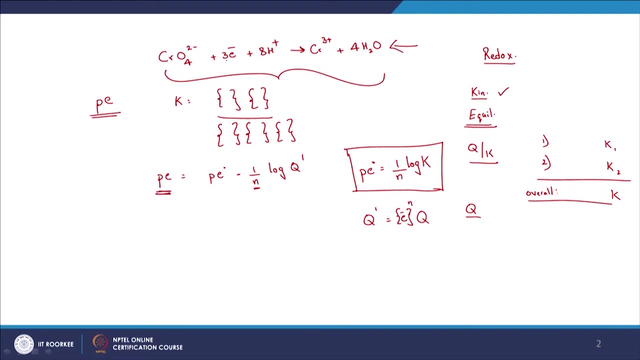 that particular, or the number of electrons being transferred. And what is n? n is the number of electrons being transferred, which in this example would be 3.. So Q dash- let me just try to write down Q dash here for this particular example. 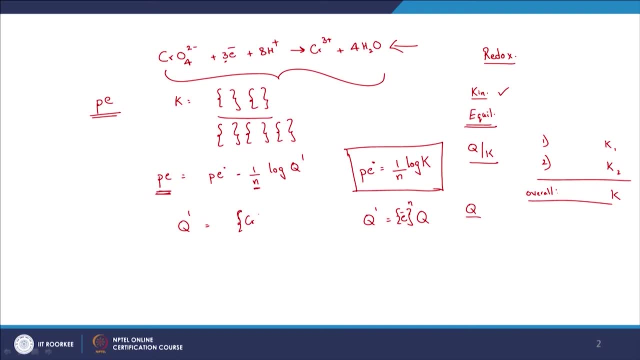 So Q dash is going to be equal to activity of Cr3+, which we usually approximate by concentration by CrO4 2-. So we are not going to have the term electron term here divided by H plus to the power of 8.. 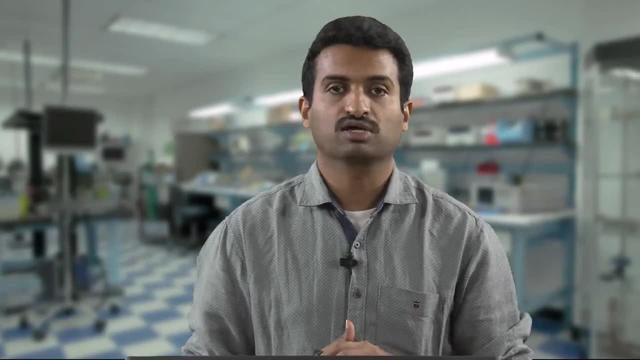 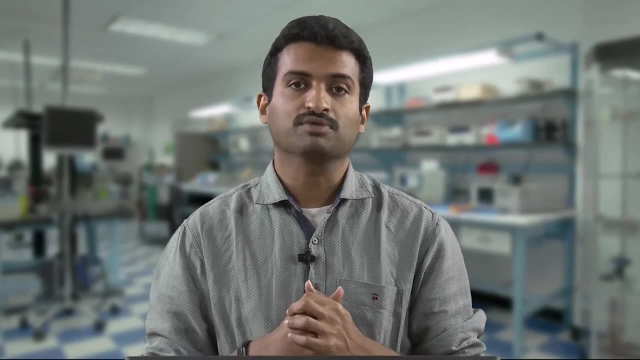 So that is Q dash here, and we know what Pe dash is, and from that we can obviously calculate Pe. So again, now we need to understand- I guess this is where we were at last time- So now we need to understand the significance of each of these variables that we have looked. 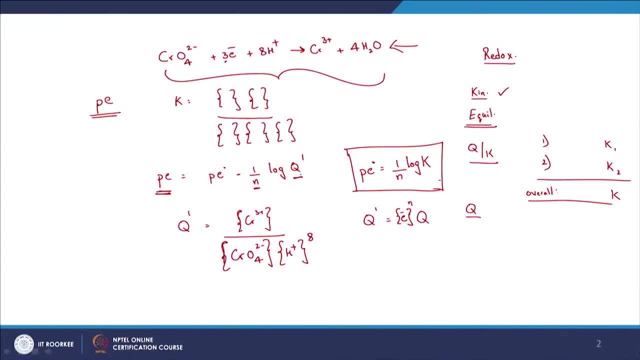 at now. So obviously Q dash gives you an idea about the current state of the system. Qu dash, we have Pe equal to Pe naught minus 1 by n log Q dash. So Q dash obviously gives you an idea about the current state of your particular system. 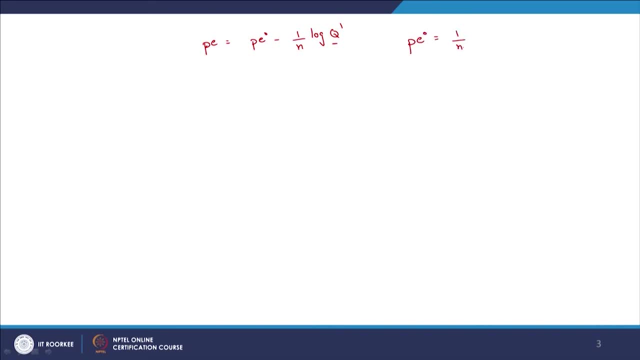 and Pe naught Right, Obviously. So in this context, we need to understand what does it mean when there is a high value of pe0 or low value or such, For that we need to understand. what does K tell us or give us an idea about? as you see, K is nothing but the activity of these. what is it now? products? 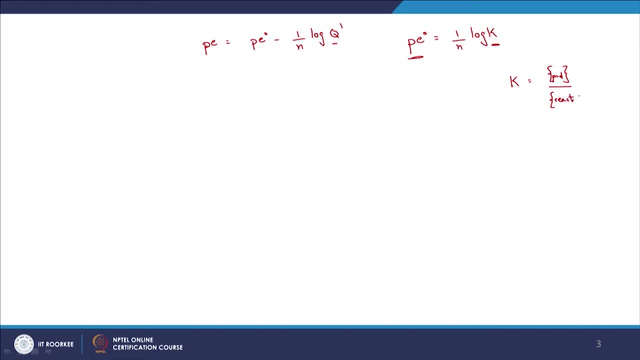 by activity of the reactants, Product of the activity of the products divided by the activity of the or product of the activity of the reactants, so raise to their stoichiometric coefficients. so this is our equilibrium coefficient. so when is this particular equilibrium coefficient going to be high? when is it going to be high when the products, the activity or the concentration? 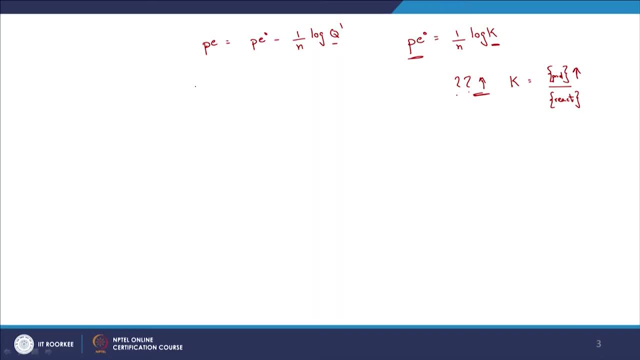 of the products is going to be high. And if you remember the way we wrote down the relevant equation, or the half reaction was oxidized form of the compound plus pe0. Electrons, or taking in the electrons goes to its reduced form A in its oxidized form. 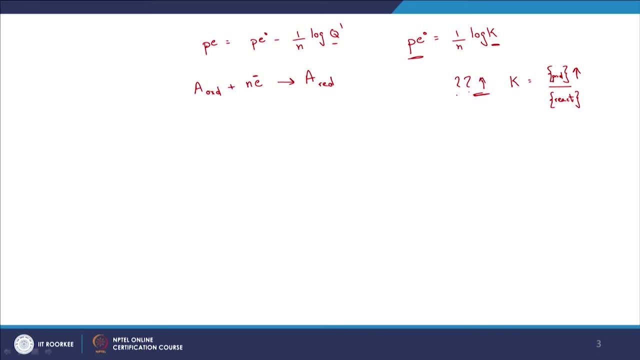 accepts electron and then transforms to it, to its reduced form, and that is what we see here: chromium, and its oxidation state number 6, O4, 2 minus 6, 2, 3. it is taking in electrons, so it is in 6 oxidation state, taking in 3 electrons, and thus the oxygen state of chromium. 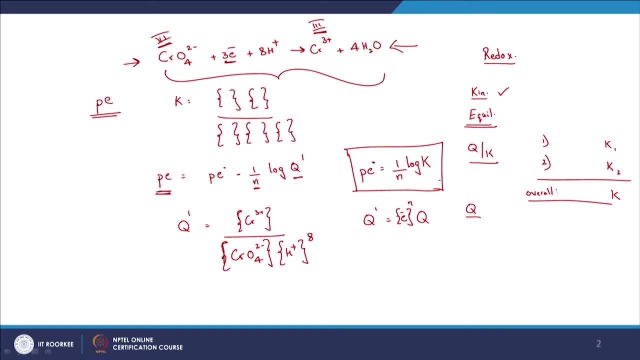 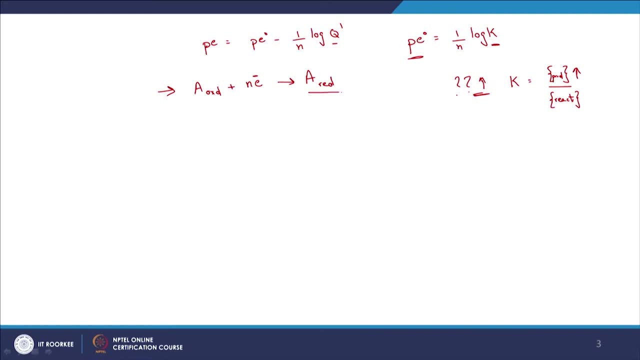 is reducing to 3.. That is what you see. Generic form is nothing but A oxidized plus the number of electrons being accepted to the reduced form of the relevant compound Here. what does it mean now if I write it down for this particular equation? so K will give me an idea about what now A activity. 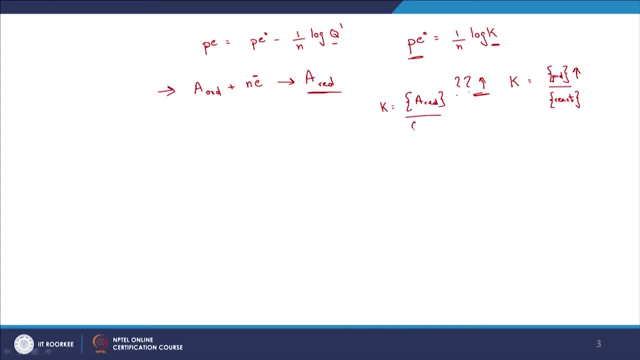 of this particular reduced form by activity, of this oxidized form in general. yes, so what does it mean? It means that the reduced form of this particular compound would predominate, or that the reaction or would want to go in this particular forward direction. so that is what a higher value of 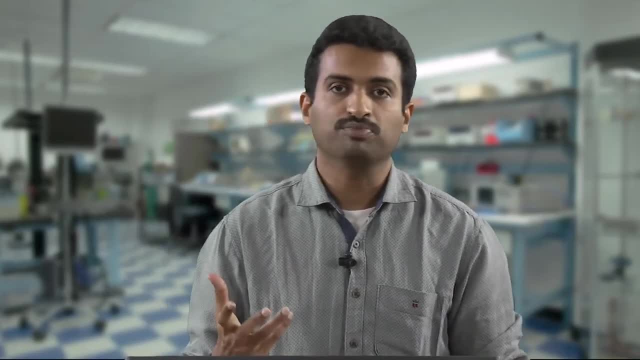 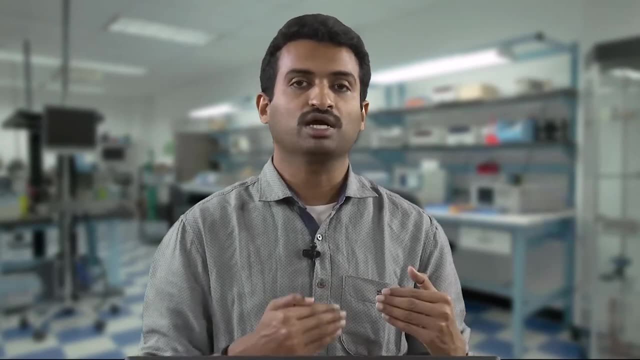 K would mean or that the reduced form would predominate. so higher value of K, more or less, as you know, translates to a higher value of pe0 value, For example, from your standard tables, if you look at the relevant pe0 values of particular half reactions. 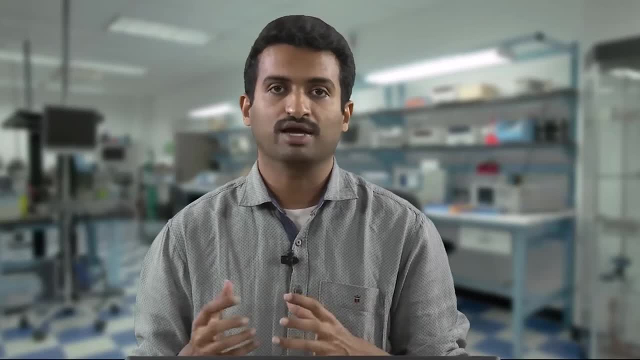 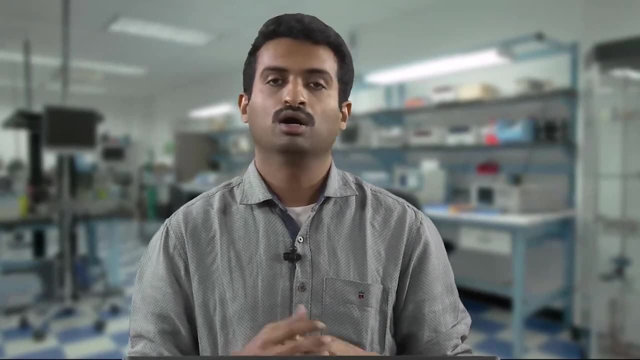 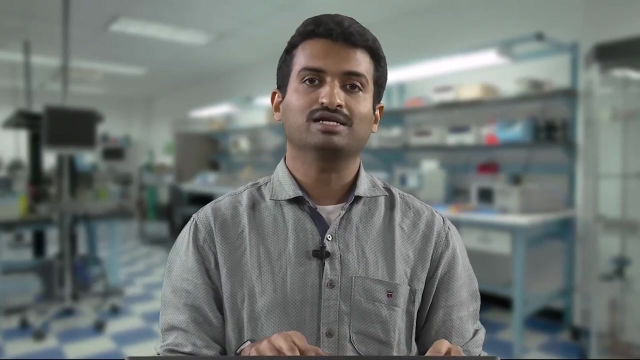 And you see that The relevant pe0 value is high. what does that mean? that it means that in for that particular system, at what you see now, the reduced form would predominate at equilibrium, or this particular forward reaction as written is going to predominate. and in which way do we write this standard? 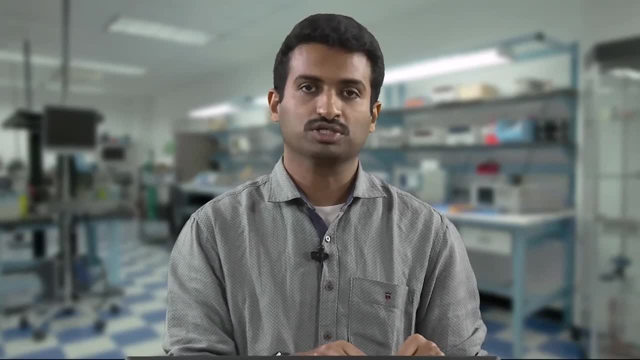 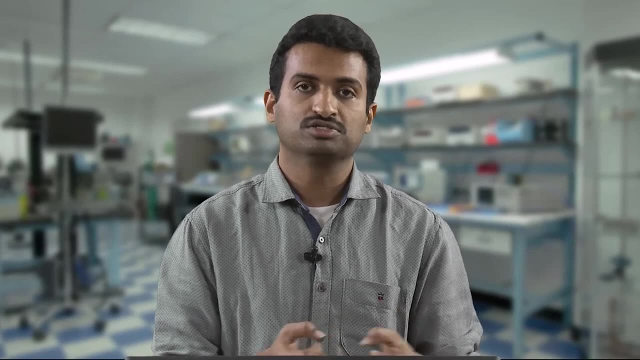 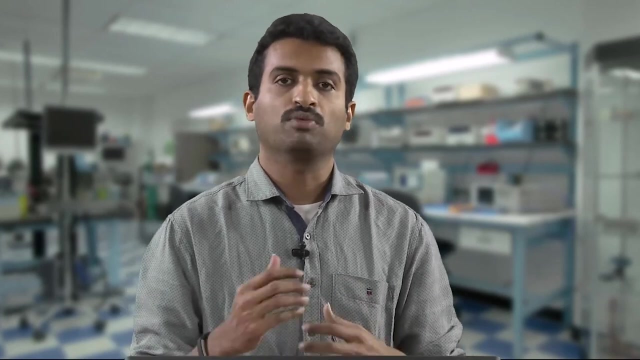 half reactions as reduction. The oxidized compound is accepting the electrons and transforming into the reduced form, so thus we can understand that this is a reduction process, And keep in mind that this is the way how the standard half reactions are written, and if you want to look at oxidation, you need to transform the or swap the reaction. yes, 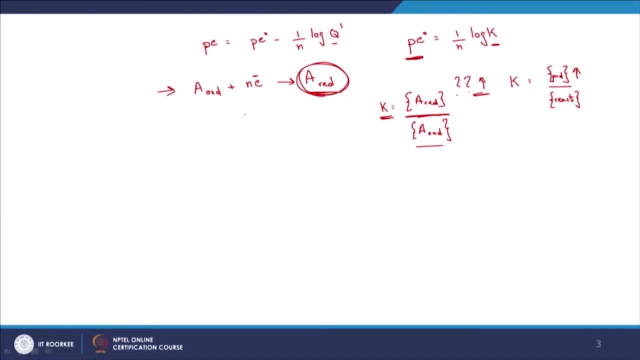 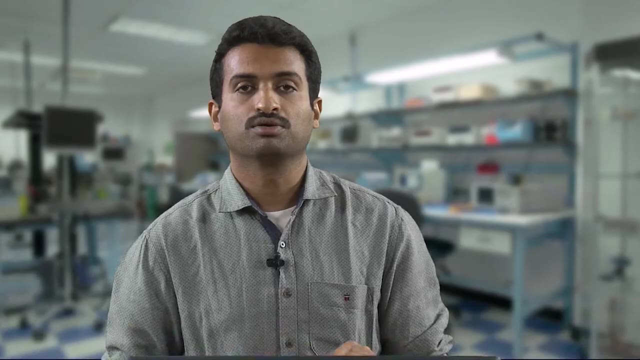 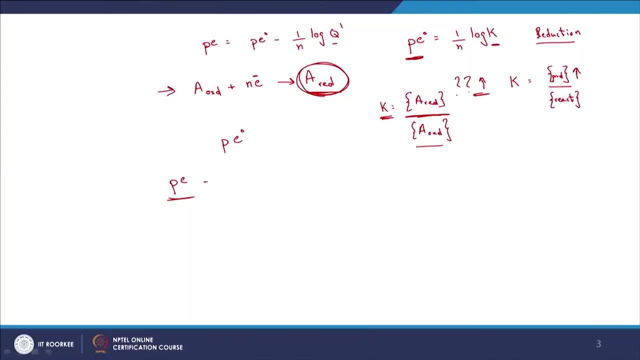 so whenever we have pe0 value to be high, that means this forward reaction or the reduction is favorable. That is what we understand from pe0. now let us move on to pe. now, how do I understand pe in relation to What have here, as in Pe0, For example? what we usually look at is Pe – Pe0. If I look, 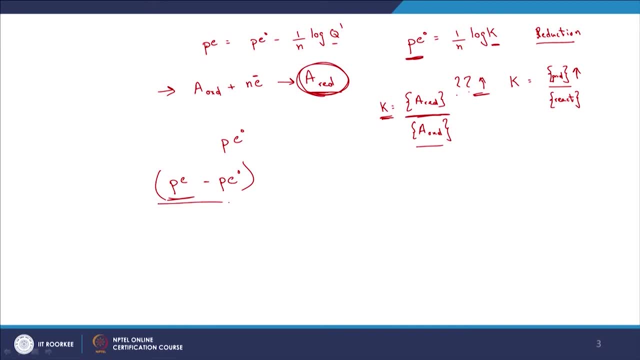 at this particular set of variables. what is it that I can understand? There are 2 cases: one when it is low and one when it is high. and what is Pe? as we know it is – log activity of electron, and that too, in the current state, more or less Pe is the negative log activity. 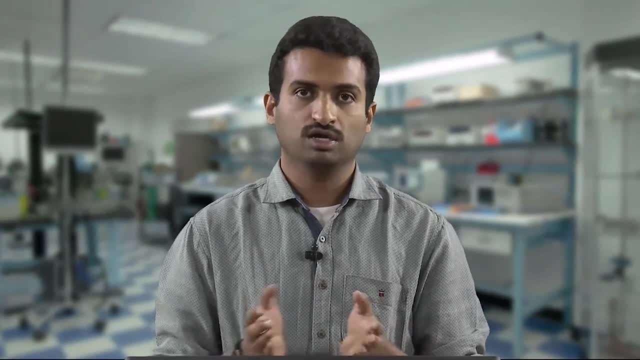 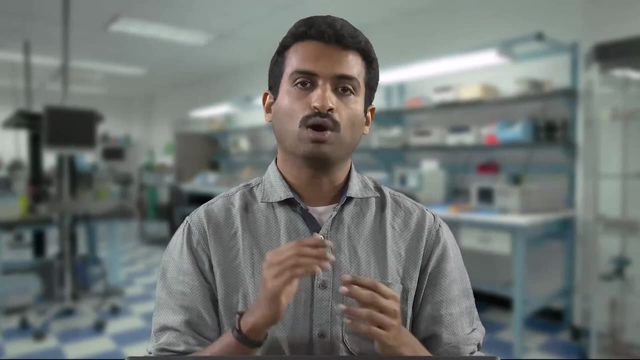 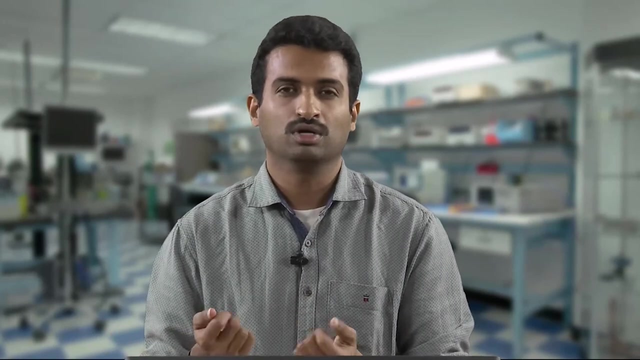 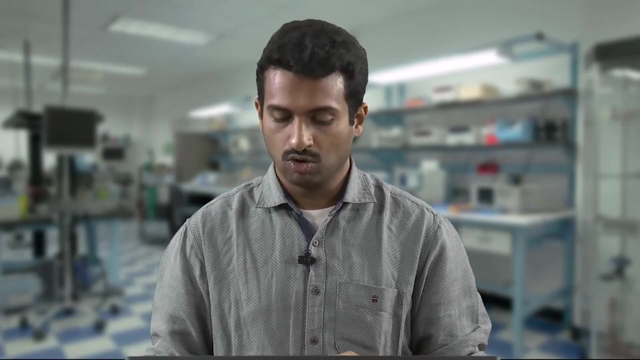 of the electron. It is similar to pH. pH is the negative log or logarithm of the H plus or the activity of H plus. Here what does a low Pe value mean? Similar to low pH value, meaning that higher H plus concentration it is negative log. that is something that is logical. 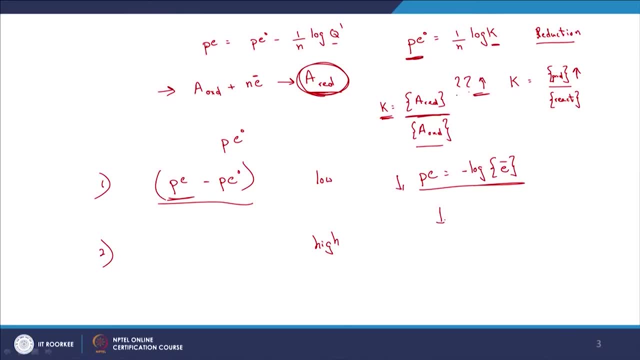 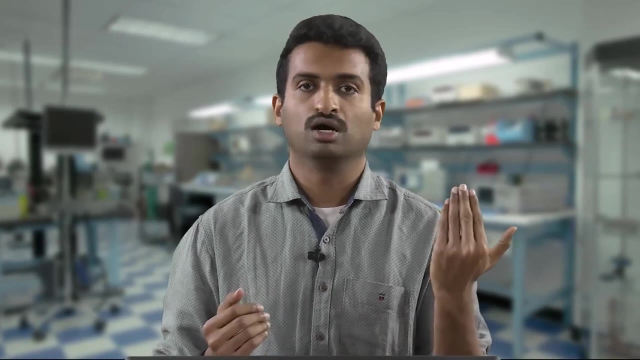 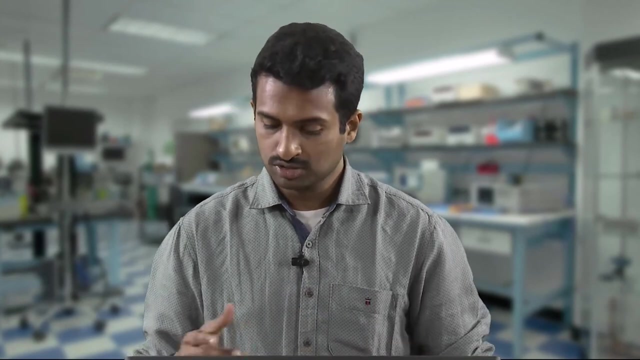 Low Pe value. a low Pe value would mean a higher concentration of H plus Higher activity of the particular electrons. if it existed in solution, As we discussed, electrons would not exist in solution. Both these oxidation and reduction processes would go in conjunction. you will never have electron pools. 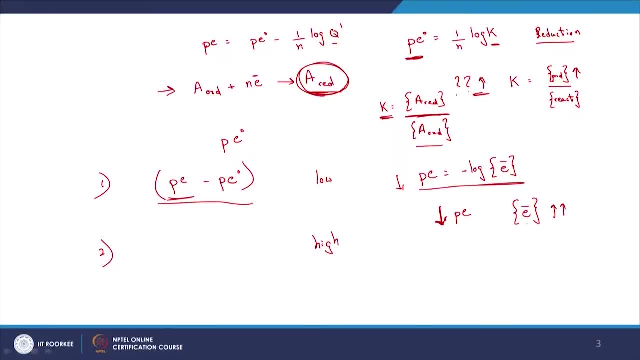 But if for this theoretical half-reaction, if the Pe is less, from this particular equation you can see that the activity of the electron will be higher. If you look at this equation, if the concentration or activity of the electron is higher, what? 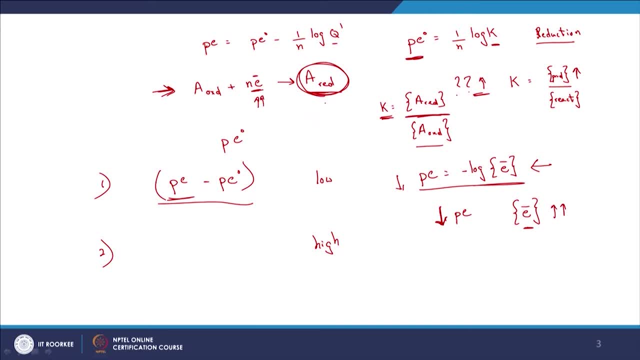 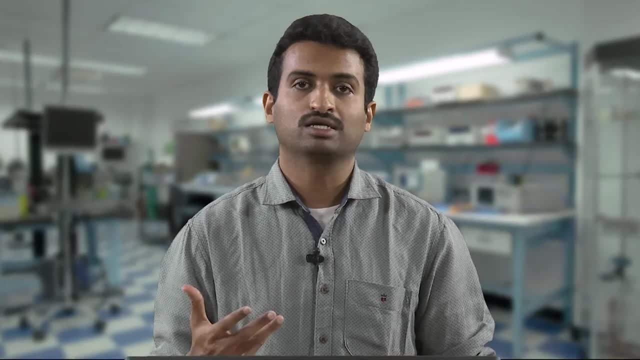 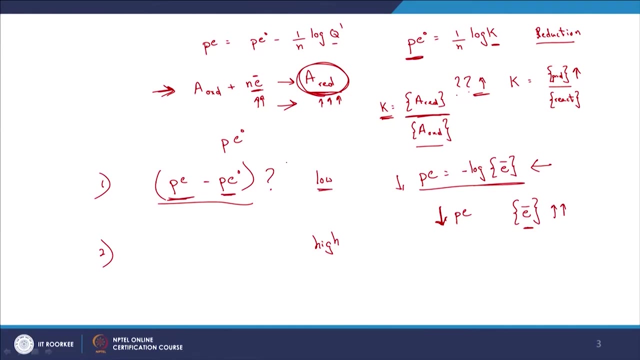 does that mean now? Then the forward reaction would be much more favorable and that the half reaction would want to proceed in the forward direction. That is what it transforms into as in. when pe then, compared to pe0, is low, what does that mean? It means that reducing 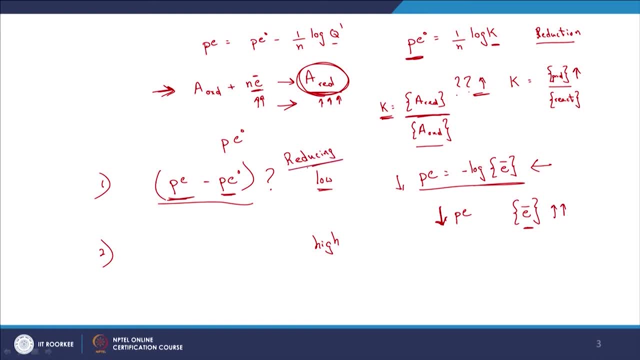 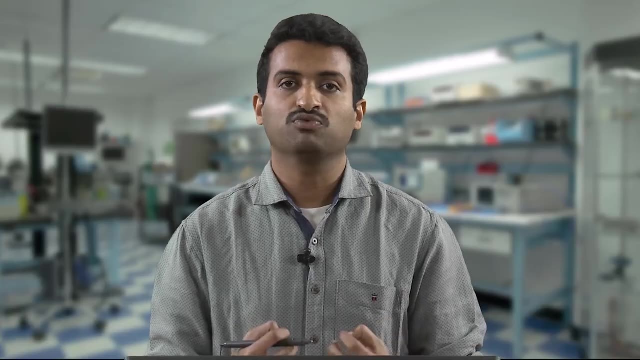 conditions prevail. Where is this from? Low pe means more or less higher concentration of or activities of your electron, as we look at from this equation 2.. It shows you that the reduced form would predominate. when would that be? When reducing conditions? 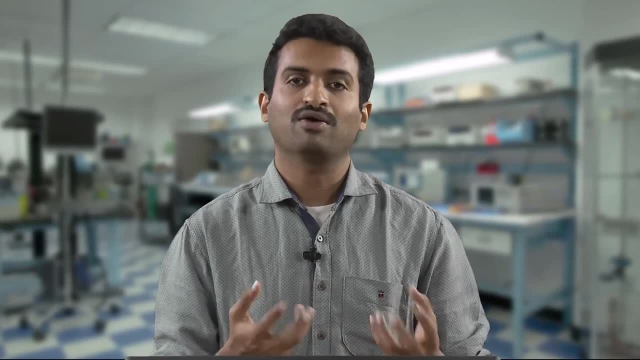 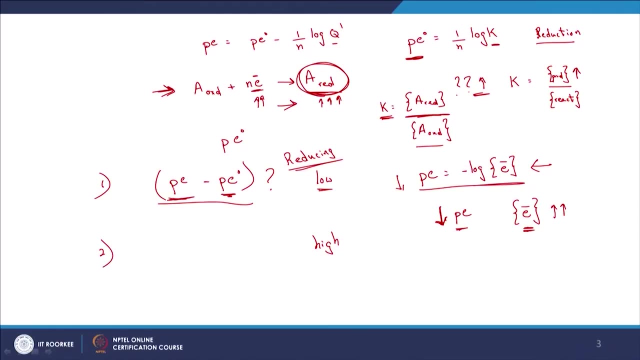 prevail reducing conditions, as in you have electrons. If you have electrons, the reducing conditions will prevail. And same case here relative to pe0, we are looking at pe, and if that value is much lower, what does that mean? Pe is pretty low and that means the 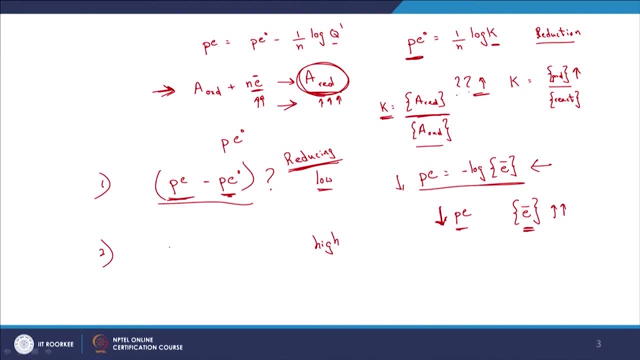 reducing conditions prevail. That is what you need to understand. If pe-pe0 is high, what does that mean? Relative to that, relative to equilibrium conditions, you see that oxidizing conditions will prevail. 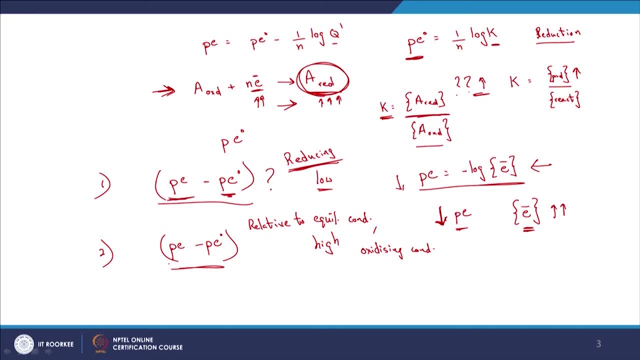 is high, so you have a high value of pe-pe0.. Finding someone is high, as well as those else pe0,嘛. test result is like this: 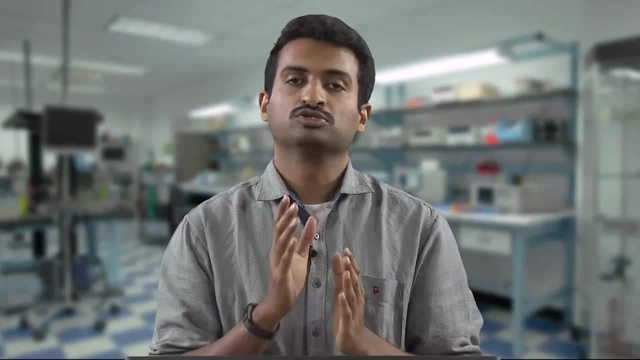 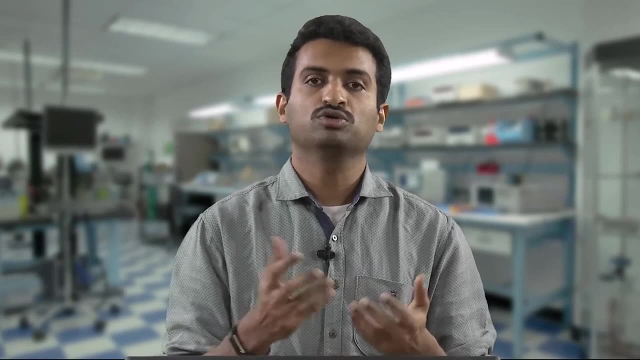 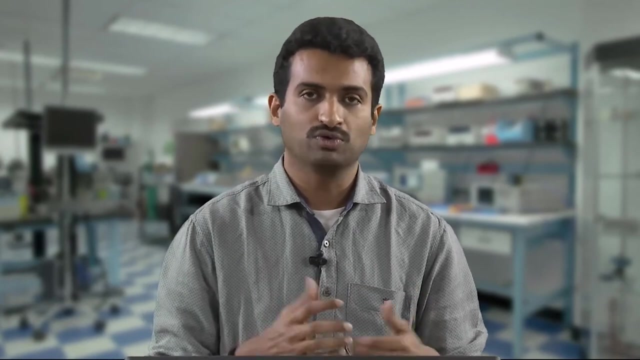 p0 gives you an idea about the system at equilibrium. Obviously higher value of pe-pe0 is going to mean that you are going to have oxidizing conditions prevail or tear off your electrons here. that is the way to understand. Here we have a graph, but before we go further or try to understand that particular graph, 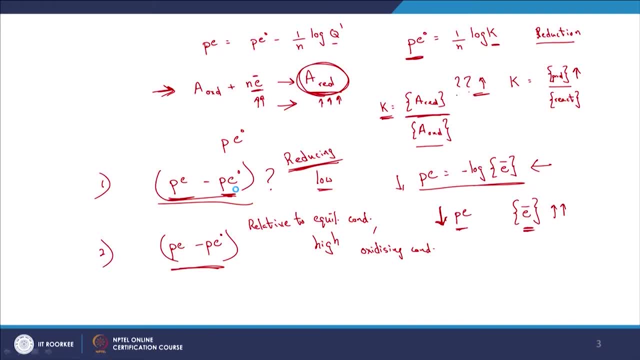 we should also be able to visualize what it is that we are trying to say. Let us plug this in in forms of what we know. Let us look at this equation again here. that is the generic equation we have here for now. Oxidized form plus the electrons go to the reduced form. 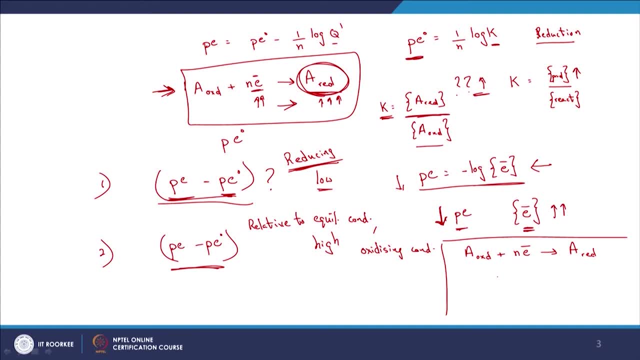 What is this similar to? It is similar to my base plus H plus going to, or my acid In this redox process, when we have the acceptance of the electron leading to formation of the reduced form of the compound. it is analogous or it is similar to base accepting the H plus. 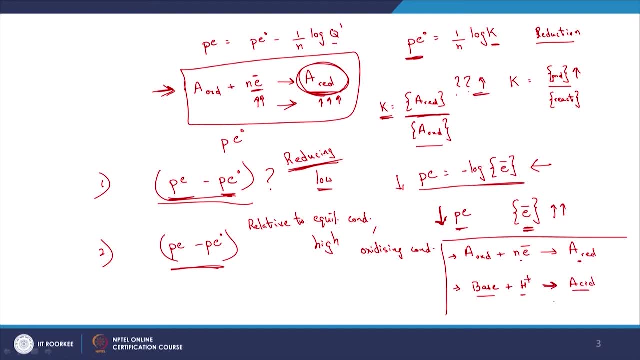 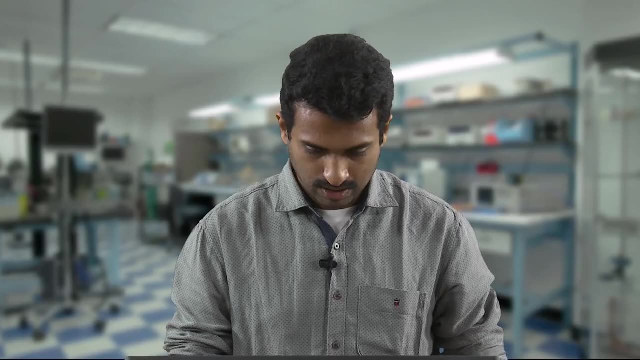 And then the acid being formed From this particular equation too. we can also try to draw comparisons between Pe, naught and the pKa values, And let us try to understand from the graph that we have in the next couple of slides, Let us try to understand the system in terms of these acid base reactions that we looked. 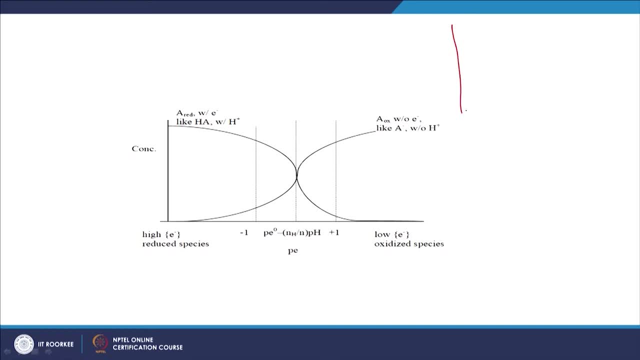 at And let us try to draw that pH pKa graph that we have always looked at. This is the concentration on the y-axis And pH on the x-axis. And what do we have? We had our protonated form, HA, and here we have our deprotonated form, or A minus. 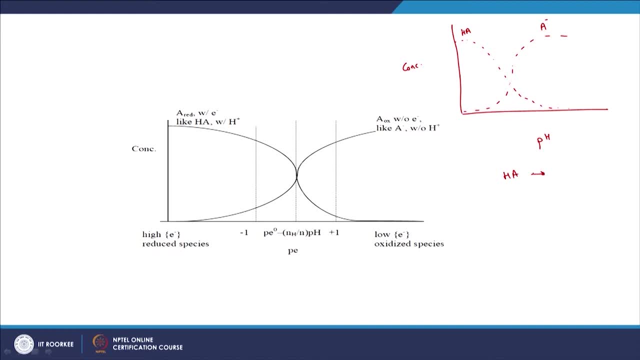 This is for the reaction where HA goes to A minus plus H plus Or, in the way that we want to understand now, H plus plus A minus goes to HA, And this particular point, when both the concentrations are equal, is pKa. What I am trying to understand, or try to help the relevant people visualise, is that 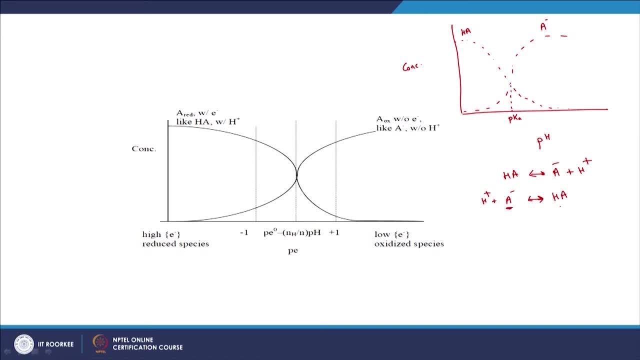 Here. let us say: this is the K compound without the proton And this is the compound with the proton. Similar to that. what we are saying is the equation that we have electrons being accepted by the compound without the electrons, compound with the electrons. 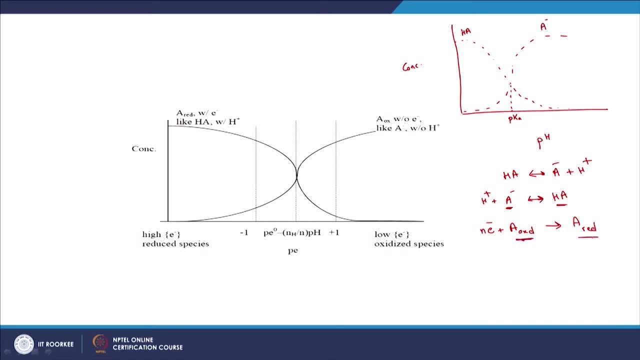 So here, A oxidized is the compound without the electrons, A reduced is the compound with the electrons or after the acceptance of the electrons. So we are trying to draw an analogy between these two, acid base and redox process. but it helps you in understanding this relevant figure that we have here. 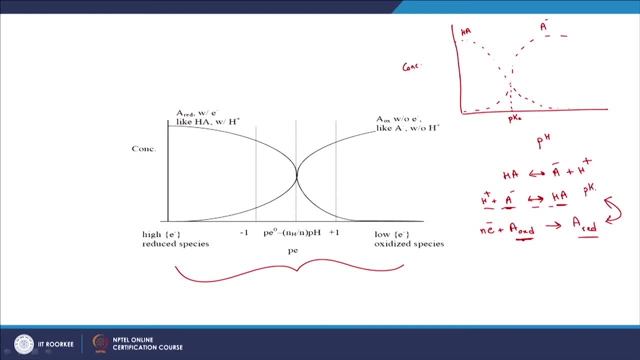 So in this context again, if you remember, we had our pKa acid dissociation constant, at least for this particular reaction. So again, the concept is similar here. So here again we have concentration on the y axis, and on the x axis we have pe instead. 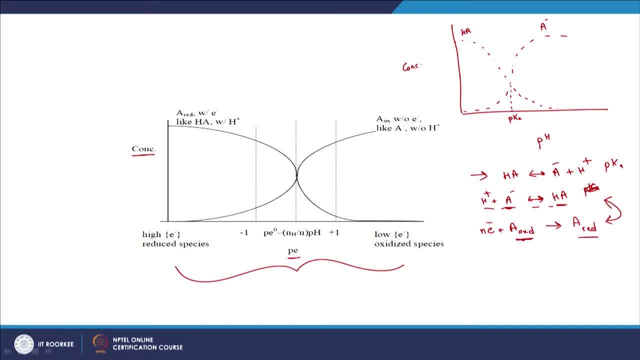 of ph. obviously for our acid base cases we had ph, So I guess this figure is a bit more detailed. so for now I guess this particular point is going to be pe0 now. So we are going to look at when this particular set of variable is going to be worthwhile. 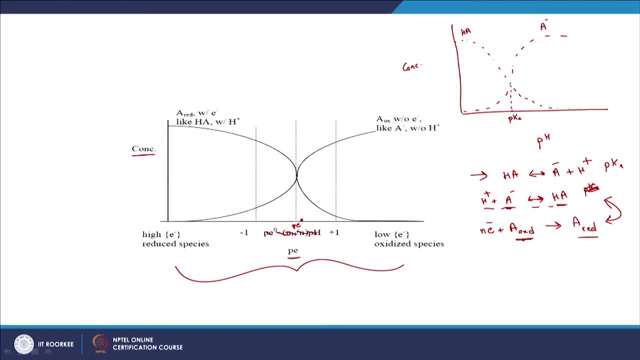 but for now we are going to consider this point to be at pe0. So again, keep in mind that this is similar to your pKa for your particular case of acid base. So again, you have concentrations here, pe and let us say pe0 is the case when, obviously, 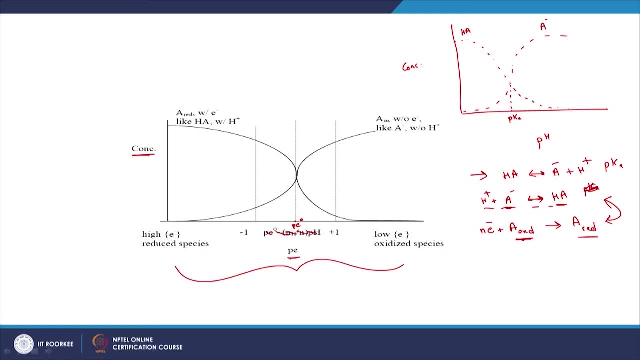 both these compounds would be at the same concentration. So let us try to understand that too. So we have: pe is equal to pe0 – 1 by N log. Okay, And what is Q dash for this particular reaction? A reduced form by A oxidized form. 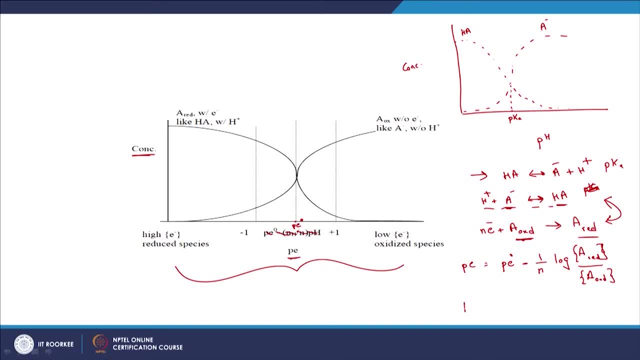 And, if you remember again, this, I guess, is similar to pH, is equal to pKa – log activity of HA by activity of A- Again, I guess it is Okay. So this is the Henderson-Hasselbalch equation that we looked at with respect to our acid. 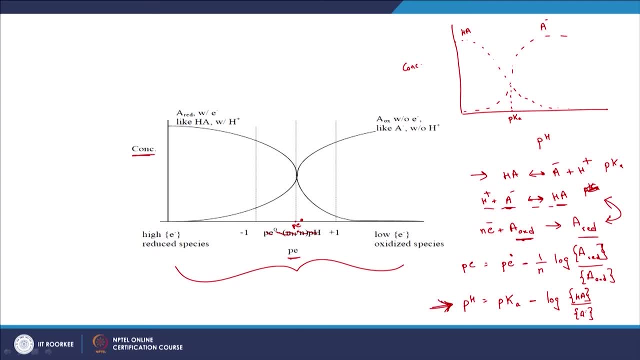 base process. This was the Henderson-Hasselbalch equation, or slight modification of it. So again, look at the analogies here. I guess. So A reduced, as in compound with the electron by the compound without the electron, and here compound with the proton divided by the compound without the proton. 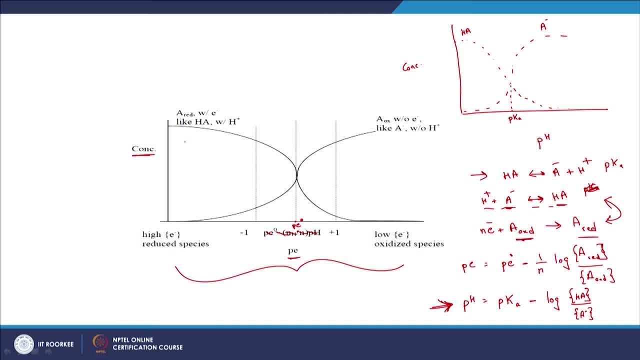 So that is what we have here and you see the analogies and similar to this here. let us say it is So. we have here the reduced form or with the electron, and this is the particular profile for that. And here we have oxidized form or without the electron, and this is the profile for the. 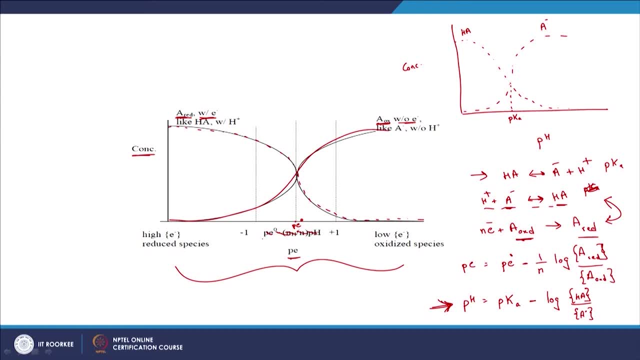 oxidized form. and you see that. what do you see? now, when pe is less than pe0, or in this region, When pe- This is pe x axis- And pe is less than pe0. Okay, Okay, So in this particular region, what do I see? which form predominates? it is the reduced. 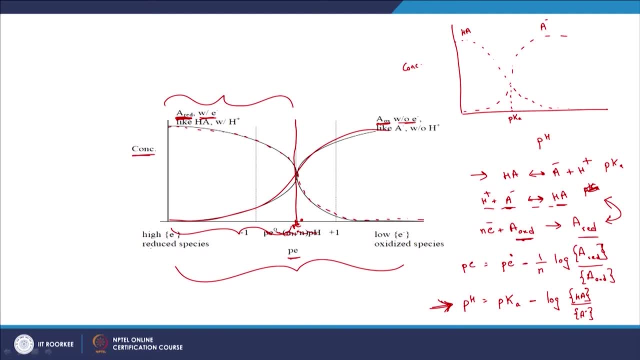 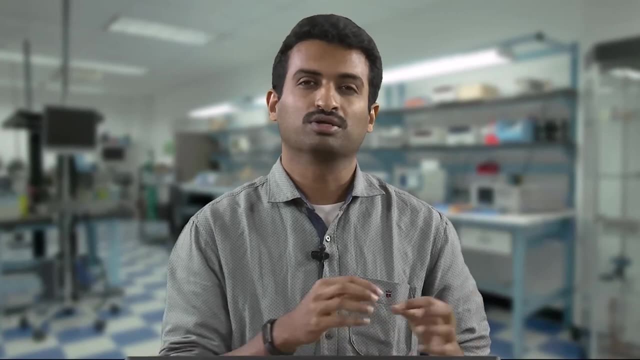 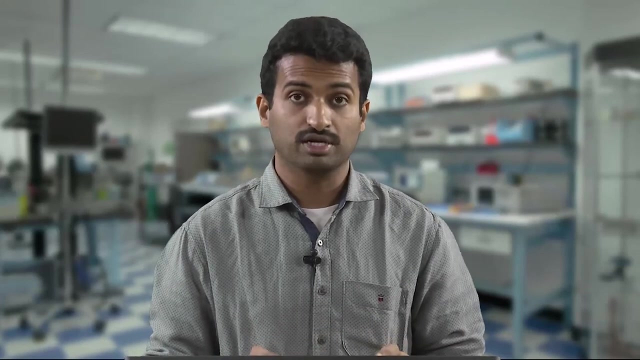 form And why is that? pe less than pe0 means high electron activities and thus reduced species would predominate. So this is visualization of the equations that we looked at earlier or the explanations we looked at earlier. We looked at a case where we had low values of pe minus pe0, and that is what we are trying. 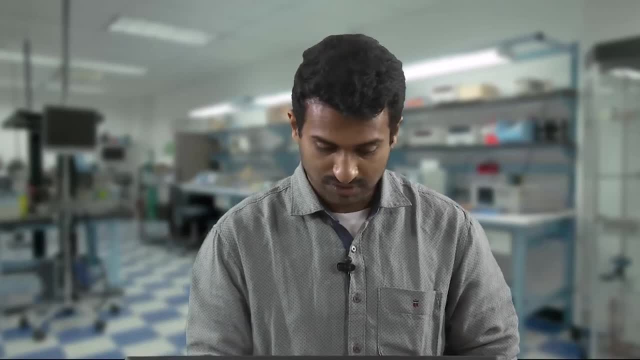 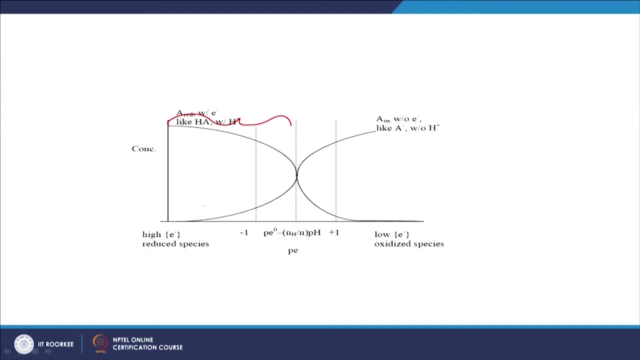 to understand or look at it here. So what do we have here? So, if you look at this particular area, what is this particular area now? obviously, when pe minus pe0 values are low or pe is less than pe0.. So this is the pe0 case, the pe0 here. 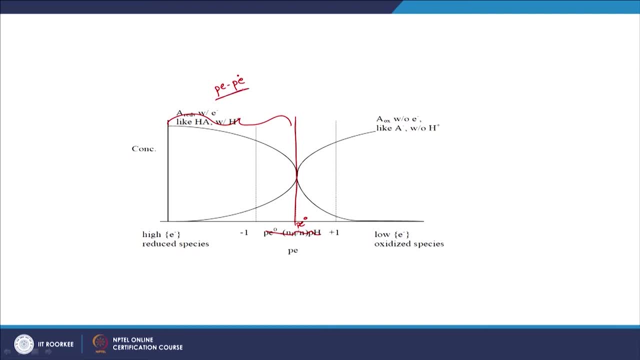 Right. So that is what you see again. When pe minus pe0 is low or pe is less than pe0, let us say obviously the we have higher concentrations of or activities of these electrons that you would expect. These are theoretical values. So obviously, when you have higher concentrations, what does it mean? A oxidized plus an electron? 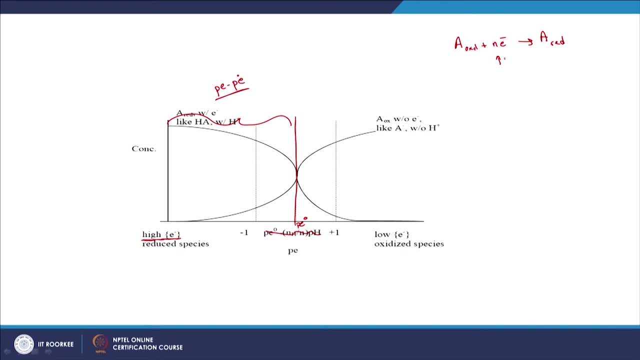 goes to A reduced. So obviously, when you have higher concentrations of these electrons, what does it mean? you will have higher concentrations of the reduced forms, Right? So that is what you see here. Obviously, A reduced form predominates when pe is less than pe0. 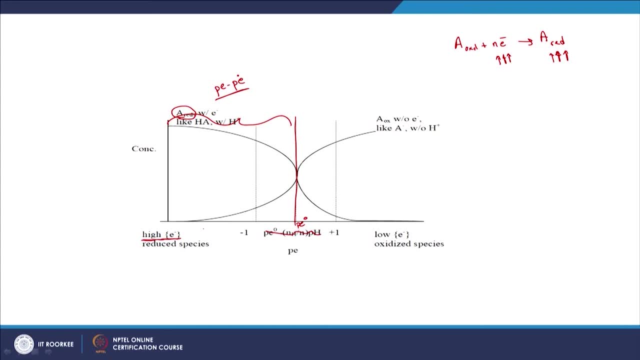 Right, So that is obviously the take home message here And obviously similarly, I guess, in that region where we have pe is greater than pe0.. Right, What do you see here? or when pe minus pe0 values are high, What do you see? obviously, 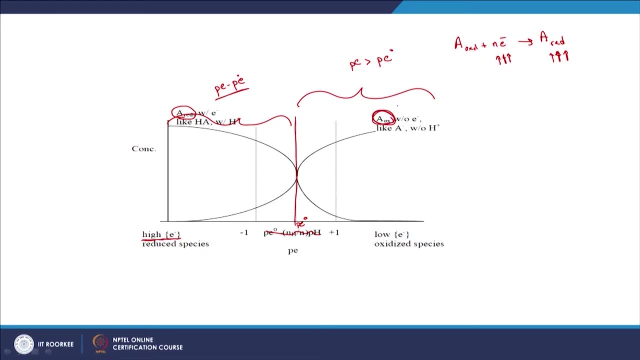 Right, You see that A oxidized form would predominate. Yes, So obviously, when would both these? A reduced Ah Activity would be equal to the activity of A oxidized Right. So if you look at that, we have the equation to be: pe equal to pe0 minus 1 by n. log what? 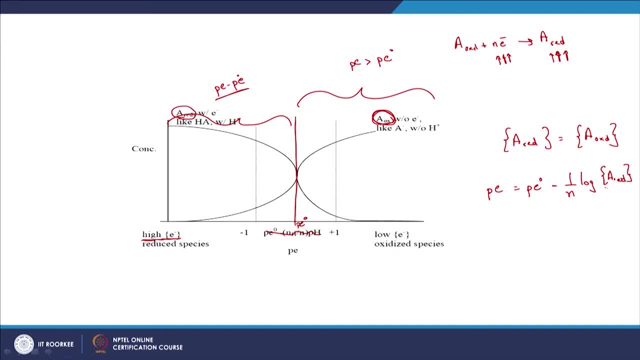 is it now A reduced by A oxidized Right? So, obviously, when will these two variables be the same? when pe is equal to pe0. Right, Then what do you see? You see that The activity of this particular reduced form of the compound will be equal to the activity. 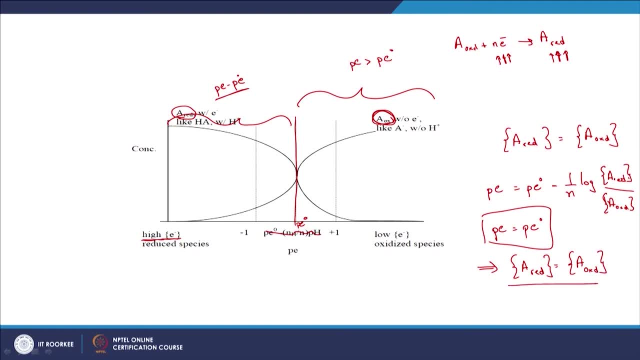 of the oxidized form of the compound Right, And obviously that is what you see in here in the graph. So at pe0, or at this particular point, what do you see? You see that activity of the reduced form is equal to activity of the oxidized form. 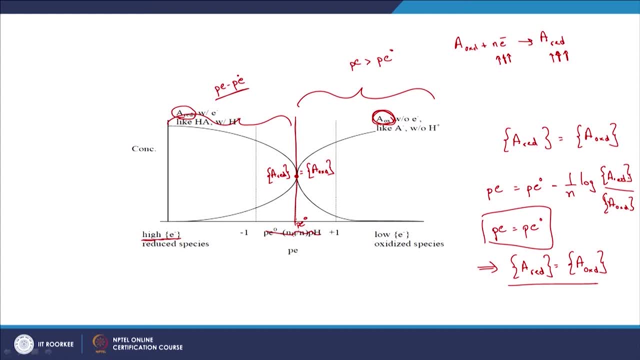 Right. And again, this is similar to our pH and pKa graph, Right. If this were the acid base relevant graph, what would it be? Here you would have HA or the protonated form. here you would have the deprotonated form. 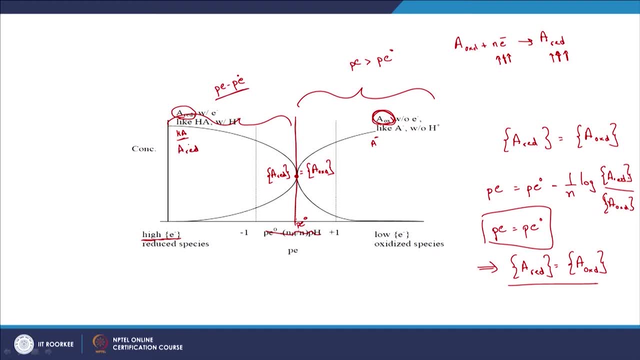 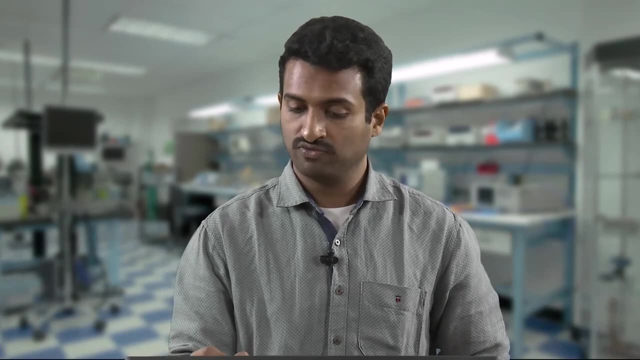 Right. So, similarly, here we have A reduced form, means with the electrons, and here you would have A oxidized form, meaning without the electrons, Right? So that is how you can help you know, understand the system, Right? So this was the case when we had a simple example of what do we say oxidized and electrons. 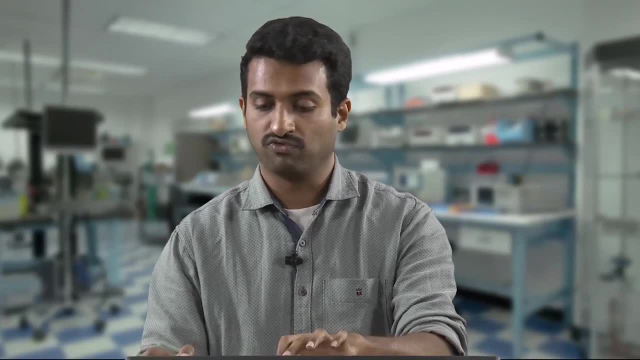 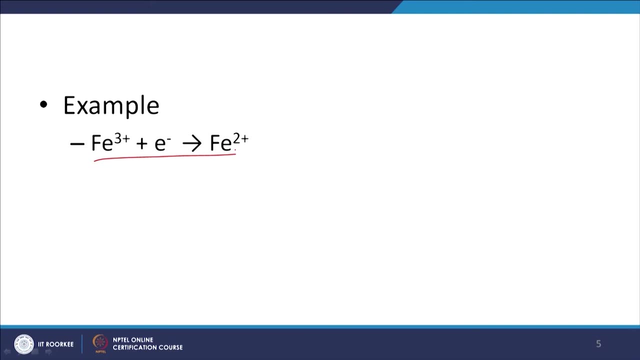 being accepted in the reduced form, I guess, Right Being formed. So now we are going to look at a couple of examples, I believe. So for this case, let us try to understand how to write the relevant aspects Right. So obviously, pe will be equal to pe0 minus 1 by n. n is the number of electrons being. 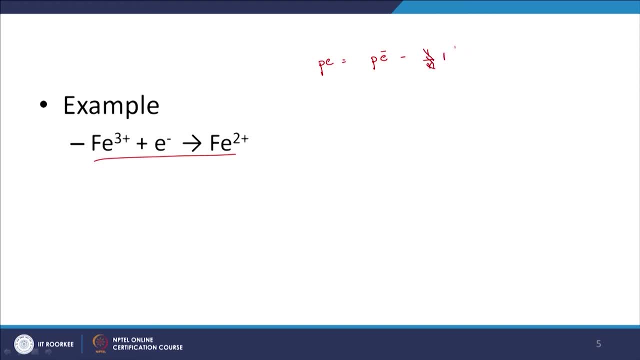 transferred here it is only 1.. So I am going to write minus 1 into log Q, dash, Q, dash, Right, So activity of Fe2+, Which is reduced form by Activity of Fe3+. Yes, So that is what you see here again, pe is equal to pe0 here, pardon me right. pe0 minus log. 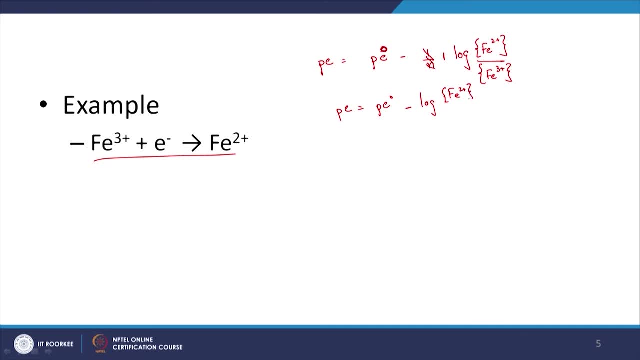 activity of Fe2+ By activity of Fe3+. Right, And obviously, again, as we looked at it from the graph, when is the when are the concentrations of the reduced form and the oxidized form going to be equal? Right, Obviously, you see that that is going to be the case when pe is equal to pe0.. 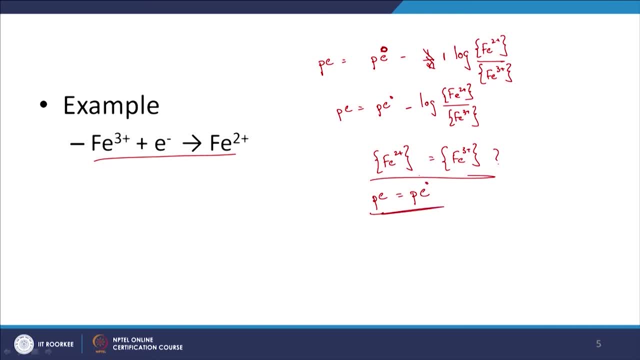 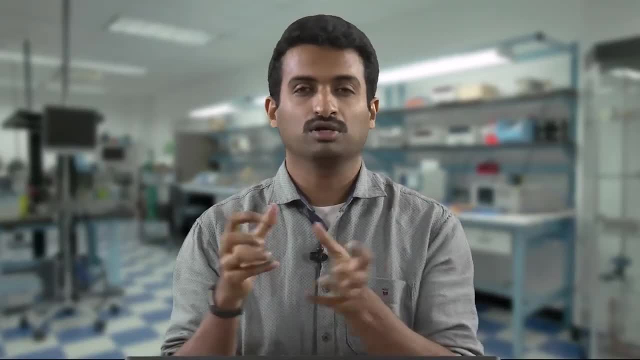 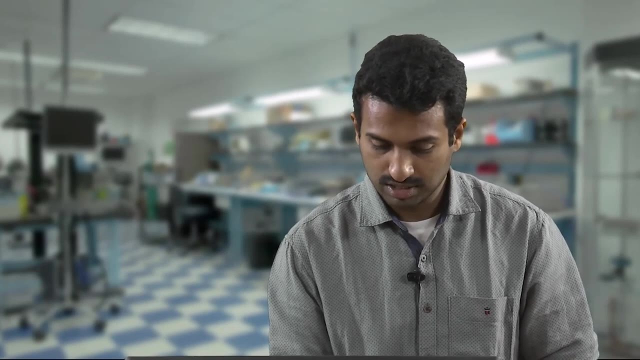 Right. So I think that is something that is obvious to understand. So, again, this is the simplest case. when you have only the oxidized form right, you know taking in or accepting electrons, and the reduced form being formed, I guess, Right, And obviously this is your oxidized form, right: oxidize, it is taking in electrons and it is. 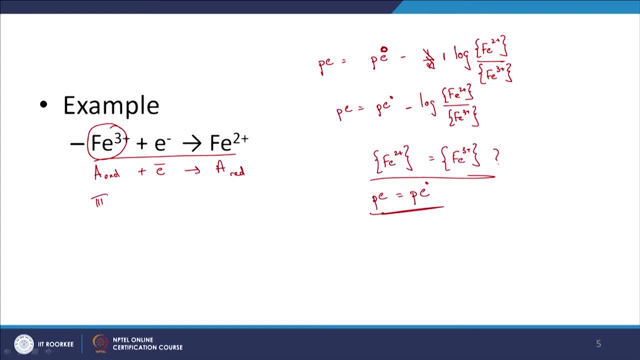 forming the reduced form. Right, The oxidized state here is 3 and because it is accepting 1 electron, it is reducing to 2. Right, I think that is a pretty simple to visualize. So let us look at one other or a couple more examples. when we also have other compounds, 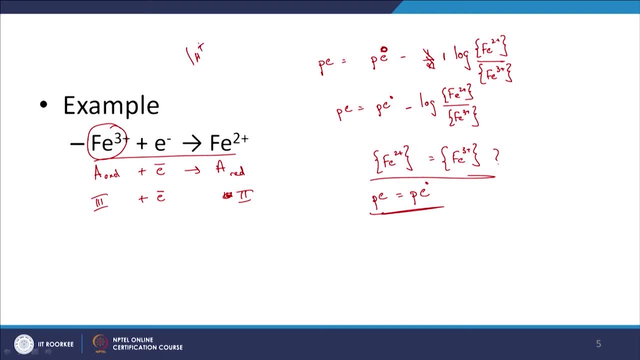 present here, primarily H+, Right, I believe the next particular example would be the one with respect to having H+. So we are going to look at a particular example or couple of examples, obviously, when we are going to have other compounds, primarily, let us say, H+. 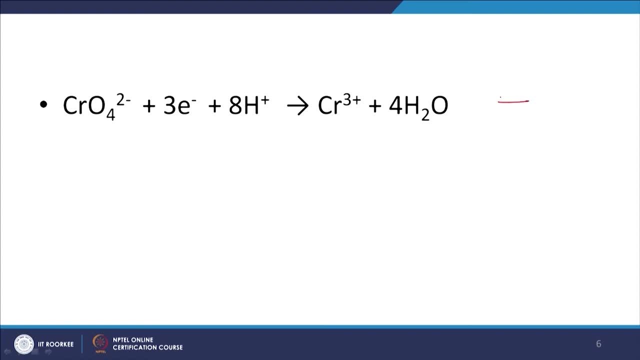 I guess. So I guess here is one example that I believe we have always looked at or considered until now. Right, We have the reduction of chromium from oxidation state 6 to 3.. Right, But I, unlike the earlier case where we had just the oxidized form and electrons being 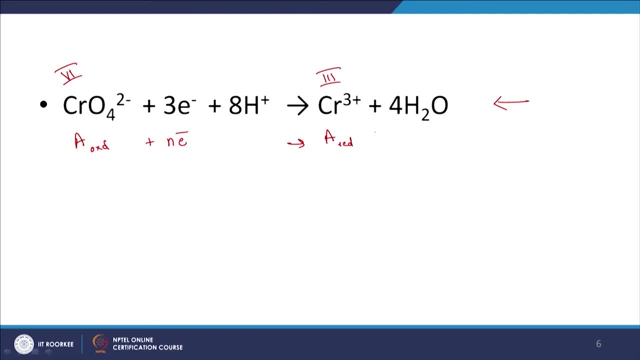 accepted and forming the reduced form- Right. We also have. what do we say H+? Here too, Right? So N is the number of moles of the electron and NH, or the stoichiometric coefficient, and H is the stoichiometric coefficient of H+. 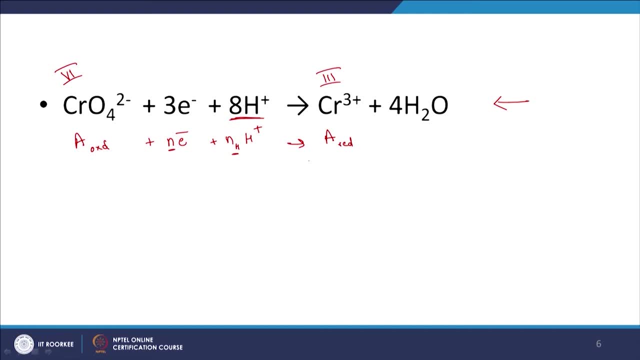 Right. So here let us say how we can modify the equation for our particular case. So let us write it down in the way that we know. So we know that Pe is equal to Pe0.. Right, Minus 1 by N log of Q dash. and what is Q dash in this particular case? 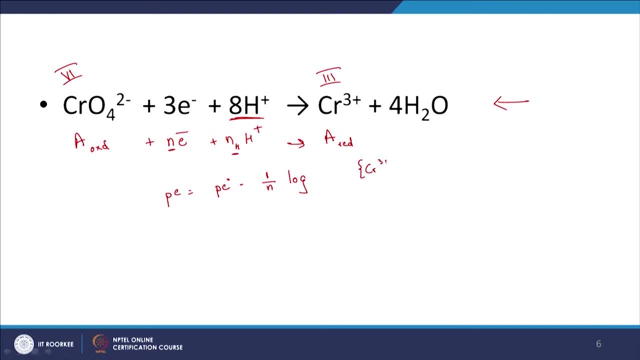 Obviously it is activity of Cr3+. By actually into activity of water dilute solutions, that is equal to 1, and activity of CrO4, 2 minus Right And electrons. we already considered that here and obviously this is Q dash. we are not going. 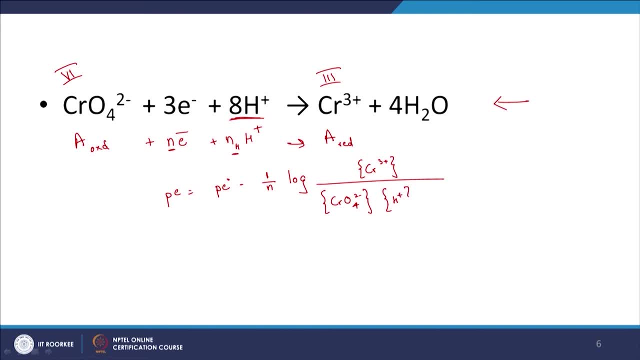 to have the electrons term here into H+ To the power of 8.. Right, And 1 by N. this N should now have been 3. Right, So I am going to say 1 by 3.. So again, Let us see how this is going to transform into Pe equal to Pe0 minus. and I am now going. 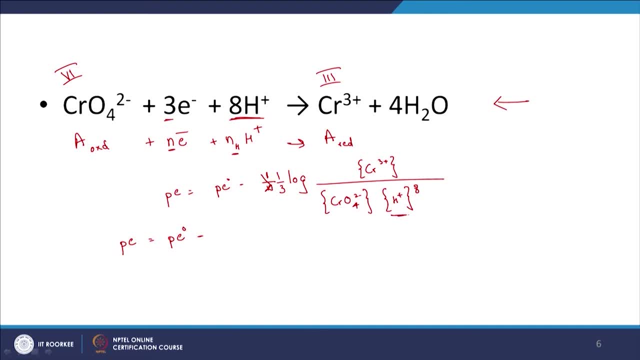 to bring this term out, Right? So what is that going to be equal to now? So that is going to be equal to minus H Right, Minus pH, Minus log H+ Right, Which is pH, and let us say, because it is denominator again, minus pH, and it is going to be 8 here. 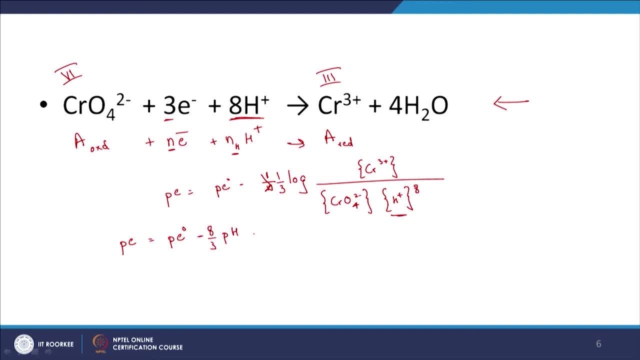 Right. So it is going to be 8 by 3.. Right Minus 1 by 3. log: Cr3 plus by CrO4, 2 minus Right. So if I want to write the generic term for this, what is this going to be? obviously Pe. 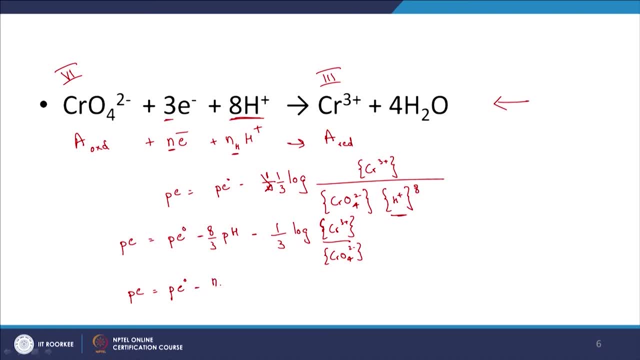 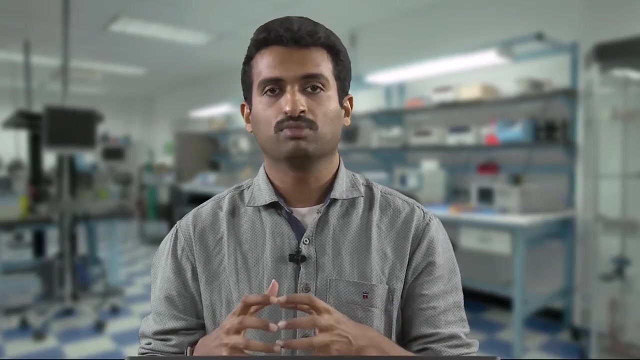 is equal to Pe0 minus NH by N into pH minus 1 by N log activity of the reduced form, by activity of the oxidized form. And the reason we express, you know, H plus outside this set of what do we say variables, is that you know, usually, let us say, when we calculate Pe, Pe0 values are 1 by N log K values are remarkably. 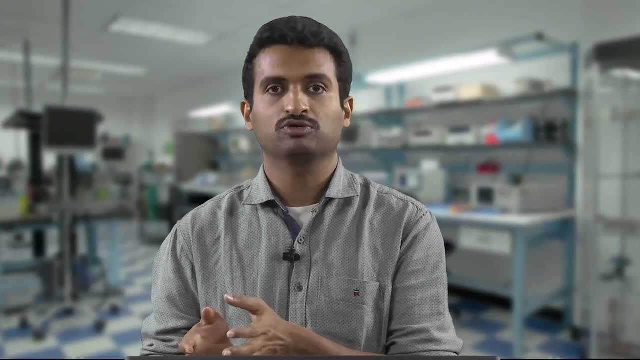 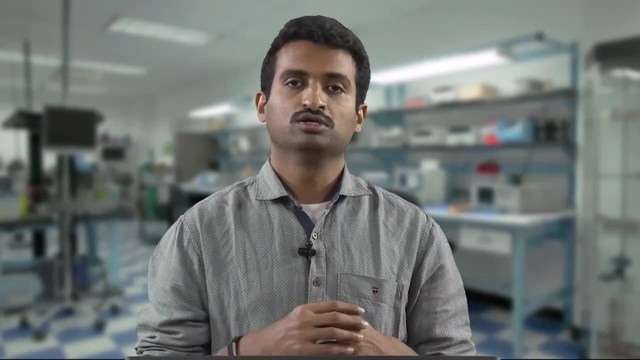 you know or not, remarkably, I guess, are significant compared to this, Q dash or log Q dash values, Right, But let us say pH, though, will have considerable role to play. Yes, Right. So again, what I guess I was trying to say is that we had Pe equal to Pe0. 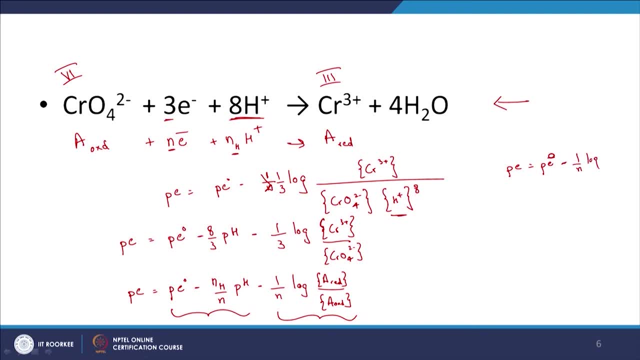 Right Minus 1 by N log Q dash Right. In general, though we have two variables here, Pe0 value will be relatively high compared to this particular set of variables, Right. But let us say though, when we have H plus involved, though, that will have a considerable 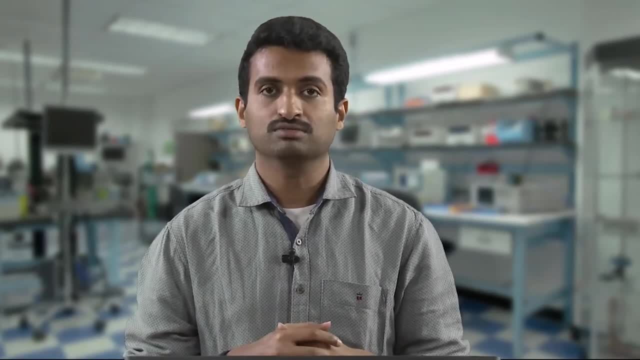 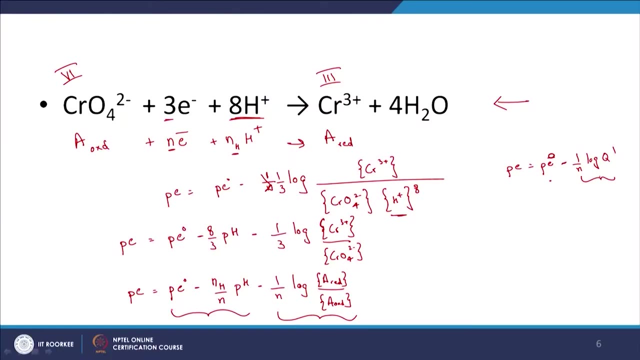 what do we say? effect on your Pe Right Or pH will have considerable effect on your reduction potential. that is what we are trying to say here, Right? So for that reason we try to express that outside this particular Q dash term and then come up with something called, let us say, Pe0W. 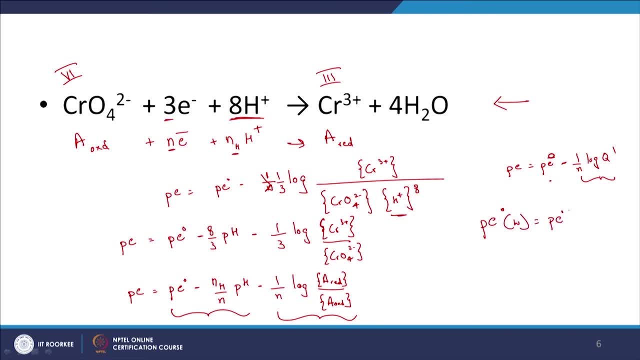 Right, Which is nothing but Pe0 minus NH by N times pH. So in the standard tables many times you will see this particular variable expressed, not just Pe0.. So obviously when you see that, that means they are talking about Pe0 minus NH by N pH. 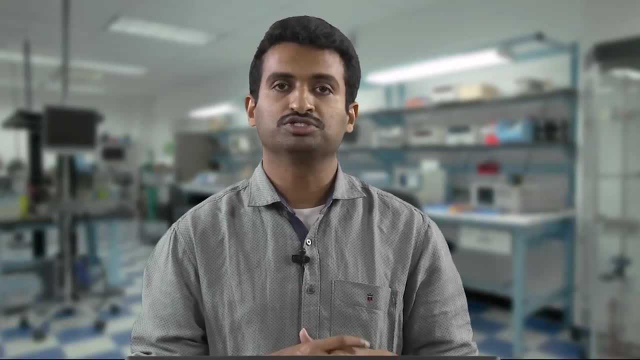 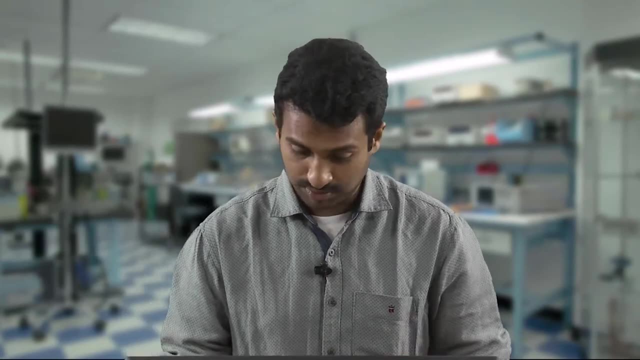 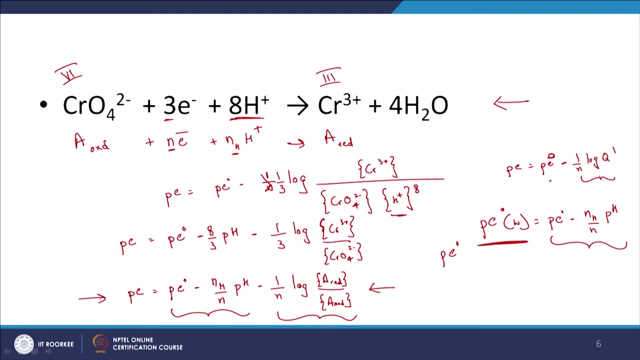 and usually at pH 7.. Right, So that helps you understand the system better, rather than having H plus inside the set of variable Q dash. Right, So that is one particular case, pardon me. So in that context, let us look at the relevant- what do we say relevant- figure with respect. 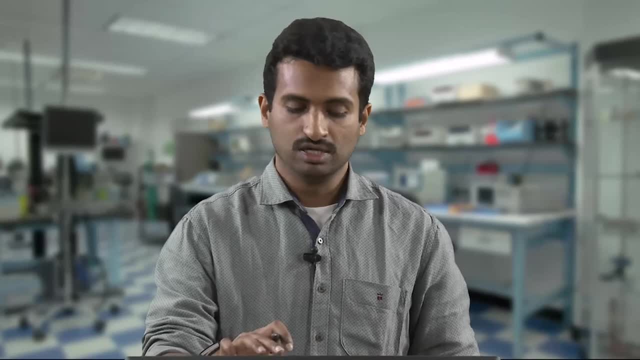 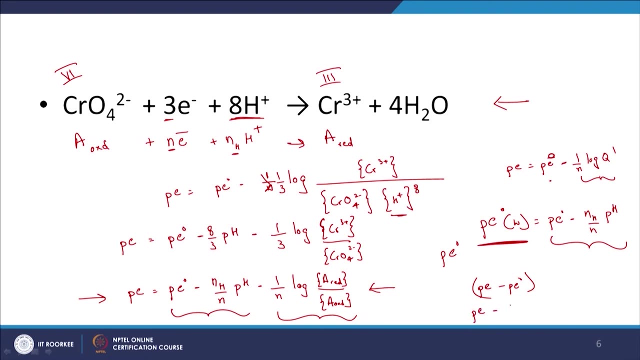 to concentration of these reduced end oxide forms and the Pe. So, again here, unlike looking at Pe minus Pe0, which was the case earlier, we are going to now look at Pe minus Pe0 minus NH by N times pH. Right, Right, Right. 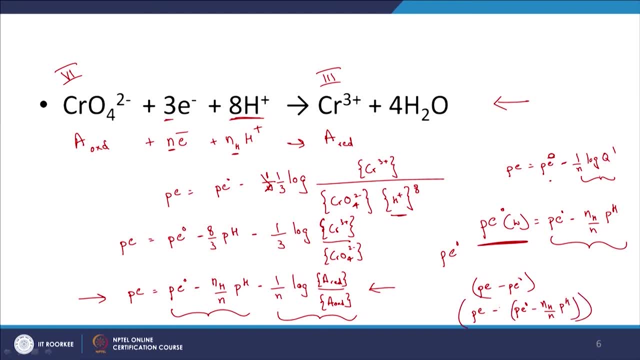 So this is what we are going to look at. So the relevant relative term or variable we are going to refer to, I guess, or the reference term, is going to be equal to Pe0 minus NH by N times pH, Right? So, and that is what we have here. 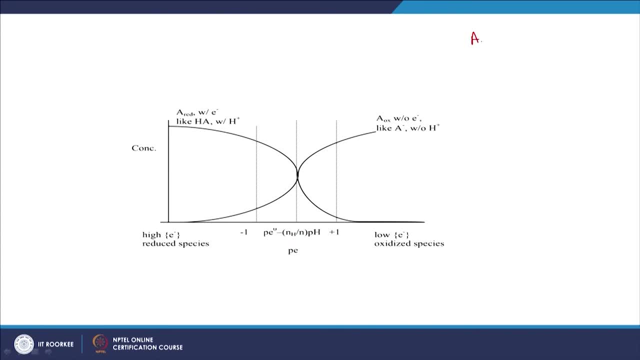 So earlier, if you remember, for that particular equation which was just A reduced plus or A oxidized plus N electrons goes to A reduced form, We did not have this particular Pe0 minus NH Right, We just had Pe0. But now when we also have A oxidized plus NH H plus right plus N electrons goes to A. 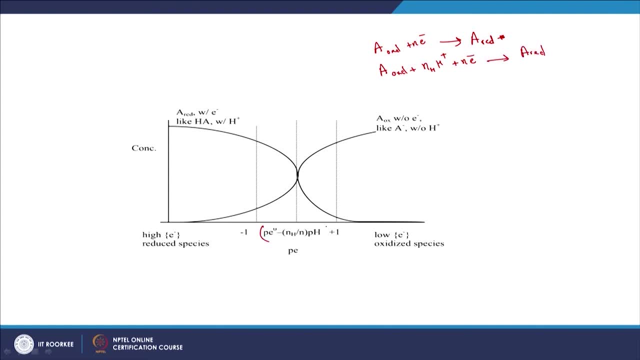 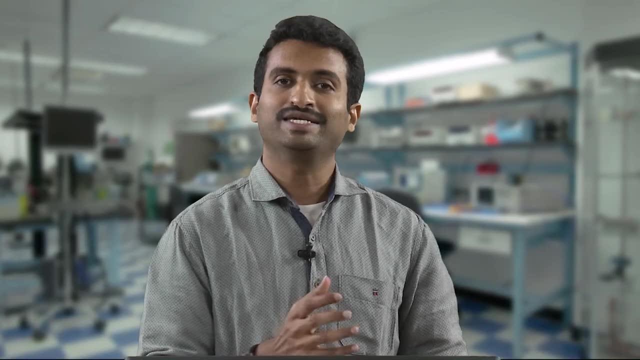 reduced forms, Right, So obviously here the reference term is Pe0 minus NH by N pH, Right, So again it is similar to that particular figure that we visualized earlier. when Pe is less than this particular set of variable, obviously what would predominate now or what? 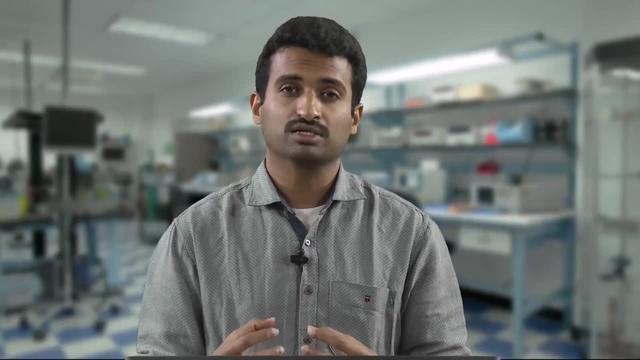 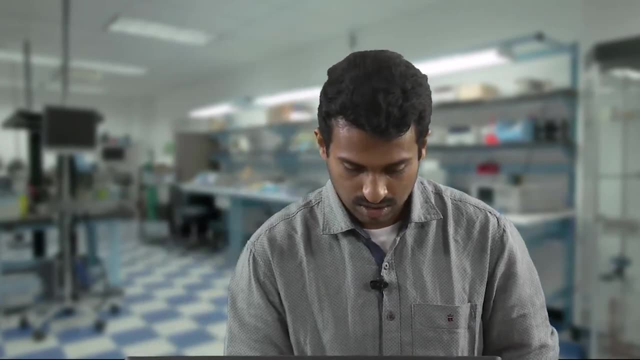 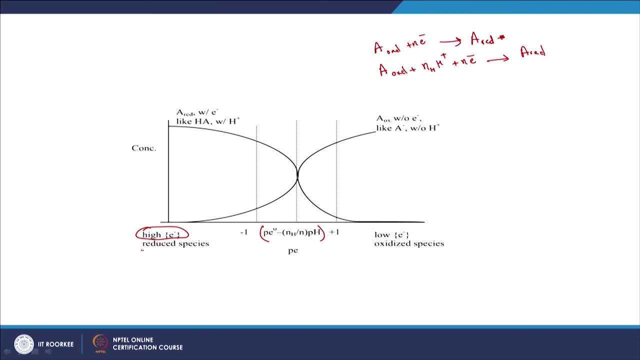 would that mean now? So Pe greater than or less than this particular reference means that Pe is very low. Pe very low means high activity of electrons. Right, That is what it means, high activity of electrons. So obviously, if electron activity is high, that would promote formation of your reduced 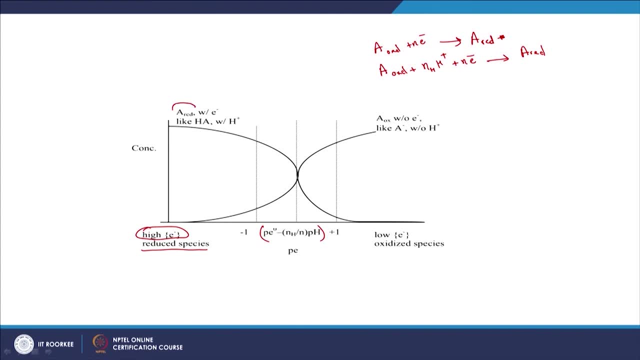 species, Right. So that obviously means A reduced form would predominate, or obviously the compound, without pardon me, with the electron Right. So obviously side, as in greater than this particular reference. what do we see? we see that the oxidized form would predominate. why is that? because low pe values, not low pe, high pe values leading. 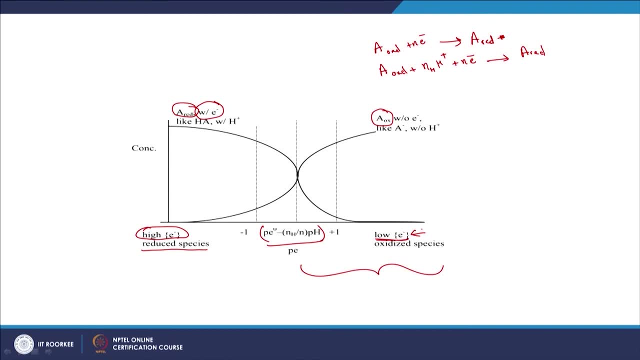 to low activities of your particular electron. low activity of your electron means oxidized species would predominate compared to your equilibrium and thus your oxidized form, or the compound without the electron, would predominate. When would your particular concentrations of these reduced and oxidized species be similar? 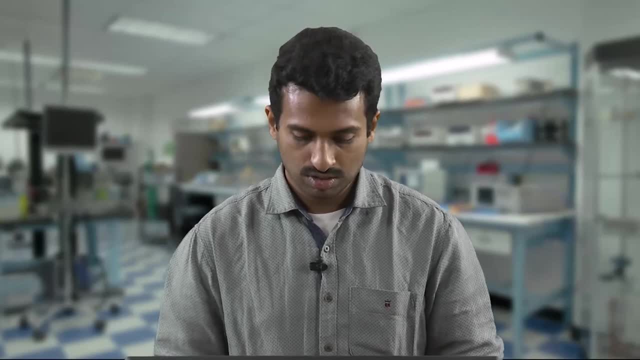 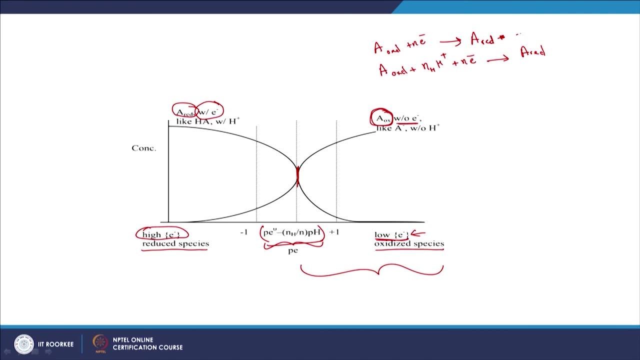 or the same. pardon me, it is going to be when pe equal to this particular reference pe0 – nH by n pH Earlier. when were they equal earlier, as in for this simple case, when pe was equal to pe0 in this case. now we have a new set of reference, that would be the case when pe equal 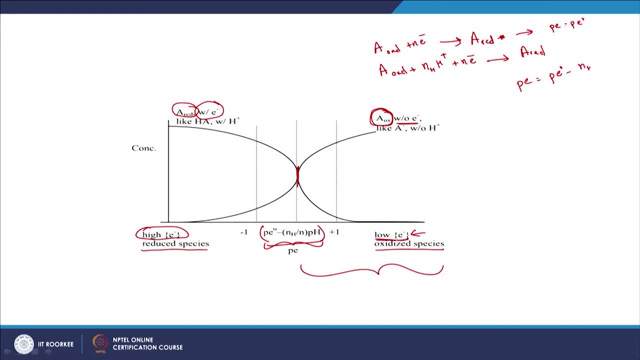 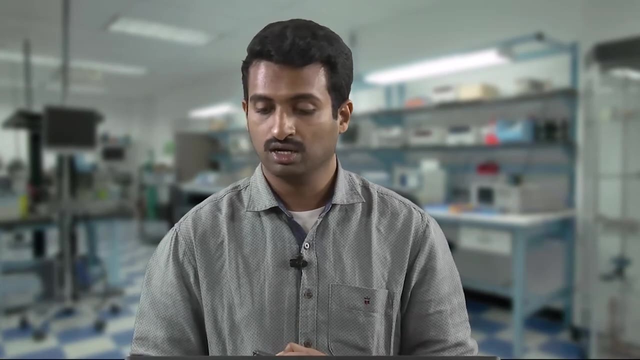 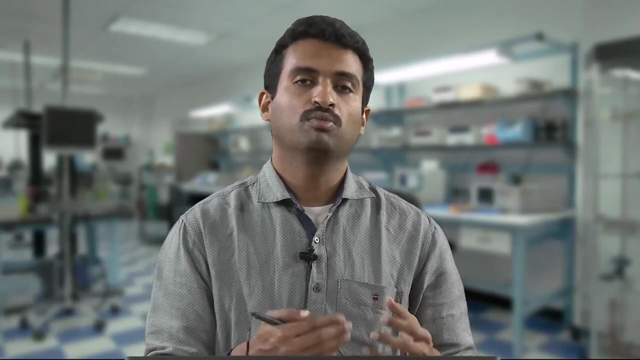 to pe0 – nH by n pH, then we would have the activity of the reduced form equal to the activity of the oxidized form. so that is one particular set of case. so now we will move on to another case when we have not just the oxidized form and the reduced form, but a few. 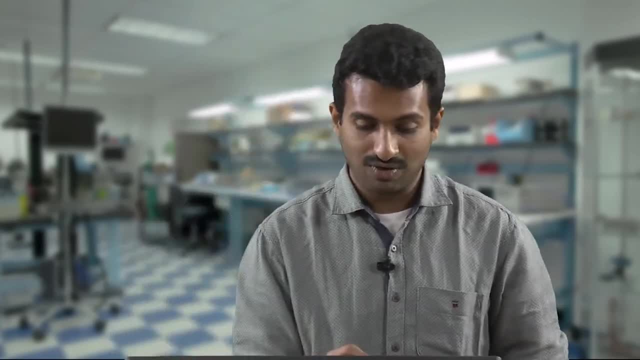 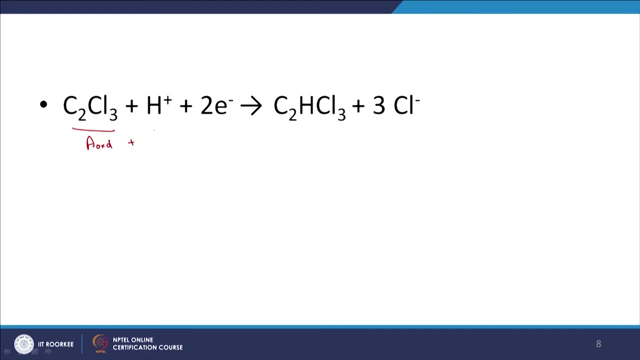 other elements. let us try to understand that. so here we have. what else do we have? we have the oxidized form here. a oxidized plus nH times H plus plus n times electrons goes to the a reduced form plus. here we also have the other elements. let us say in this case: 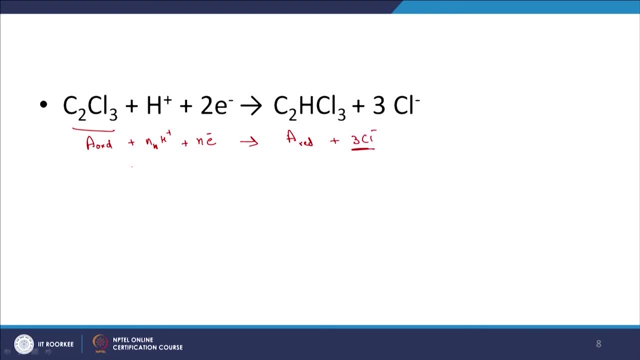 3Cl – 2. so here we need to try to understand the system. so we have pe equal to pe0 – nH by n, pH is 1, by n is 2 times pH – log Q'. what was log or what is log Q'? it is C2HCl3 into. 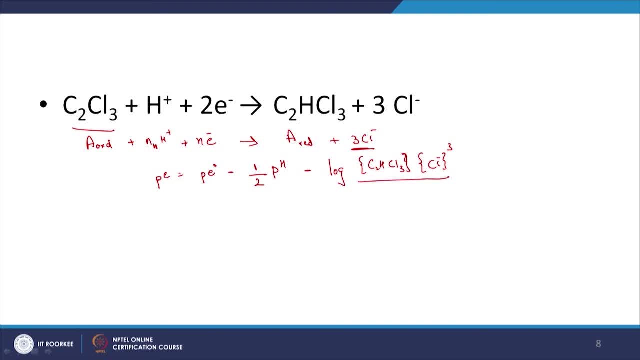 Cl minus activity raise to the power of 3 divided by C2Cl3 and its activity here. so we will just look at the simple case when our concentrations of C2Cl3. Concentrations of C2Cl3 would be equal to the concentrations of C2HCl3. so when would 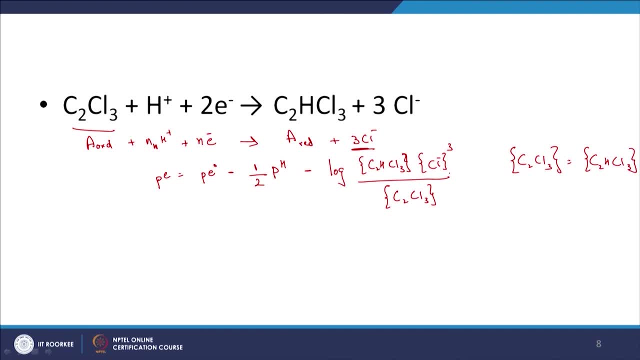 that be the case. let us try to take this Cl minus term outside. so it is going to be equal to pe, equal to pe0 – 1 by 2 pH and we are going to have – 3 log Cl minus activity. When will this particular equation be valid, when pe is equal to this set of variables? 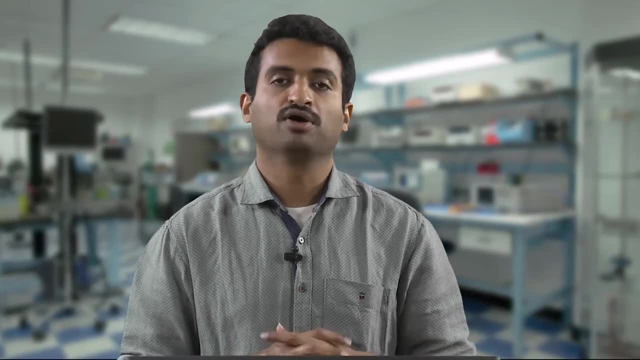 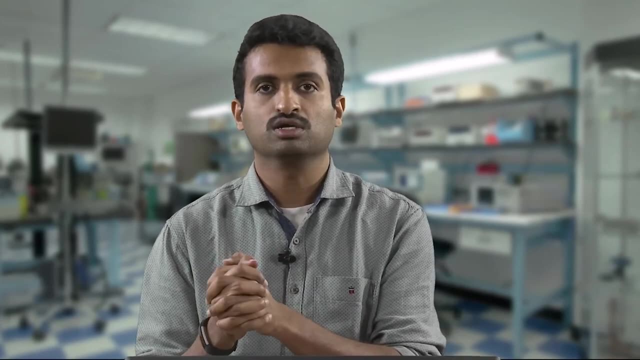 so, just for our purposes understanding, we start with the basic example, when we had just the oxidized form, accepting a few electrons and transforming into the reduced form, and then We did the Tamburian scale. We also looked at the case where we also have H plus, and now we are looking at a bit more. 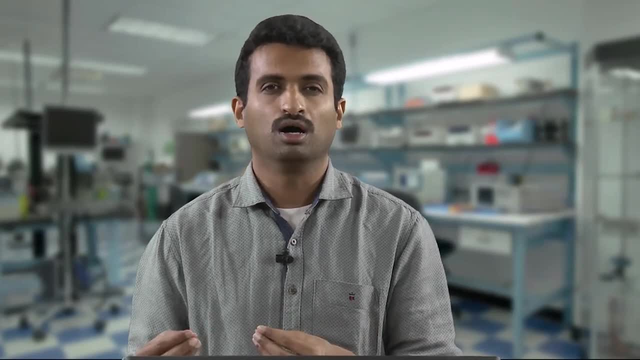 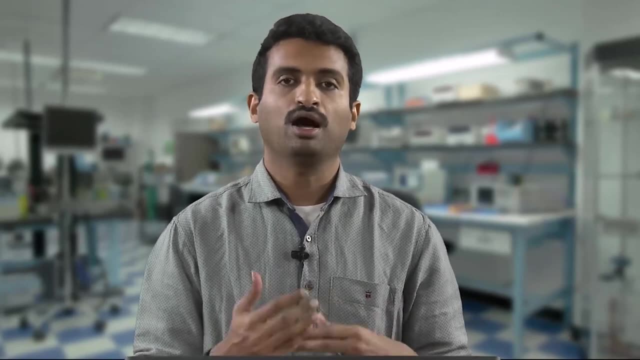 complex What we say system or the half reaction- a bit more complex half reaction, but the objective here is to be able to understand the basic equation and how you need to transform it or visualize it so that you can look at the relevant variables and understand the underlying. 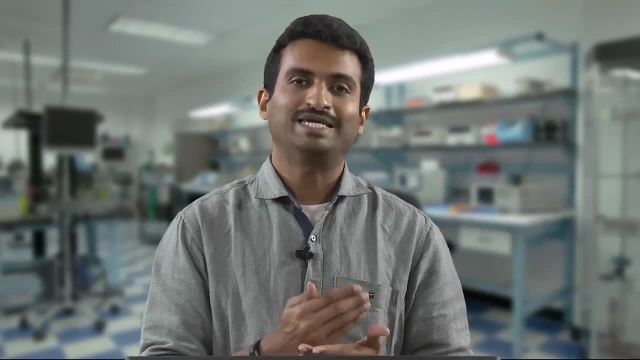 aspects And primarily, what do we understand here when pe is low or lower than your particular reference, which is pe0, the pH or pe0 –, nh by n, d0, I forget how- called pe0, so essentially the P, mine Hieroglyphs power, or lower than 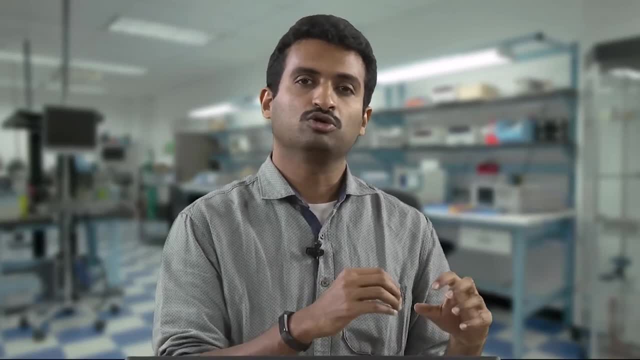 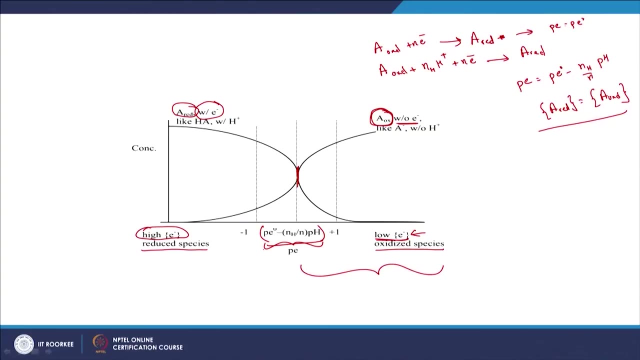 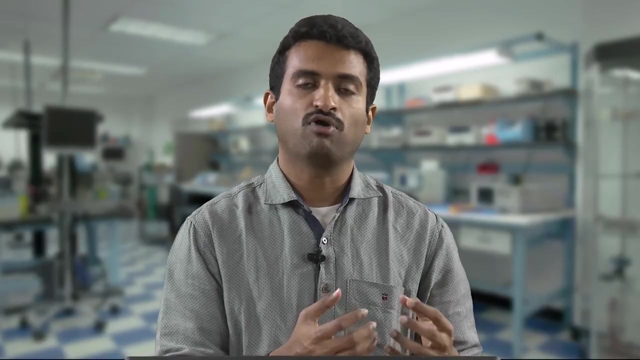 n into pH. what does that mean? that means your particular activity of electrons is high. Let us look at that equation here. so we will just summarize for today. and that means high activity of electrons meaning your reduced species concentration is going to be higher. that means a reduced form is going to predominate when Pe is less than your particular reference. 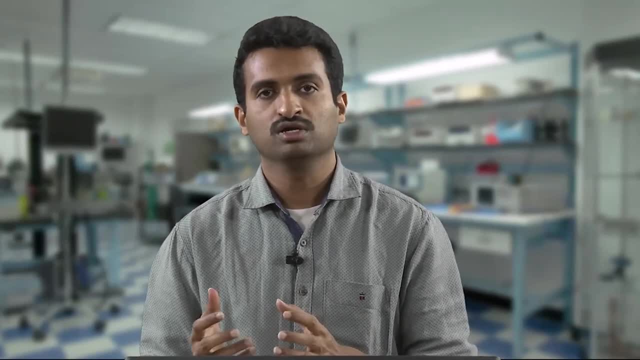 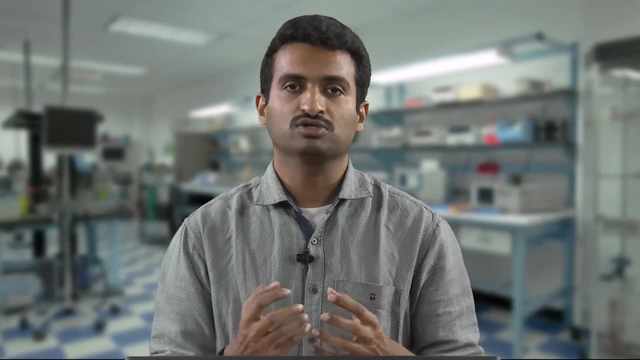 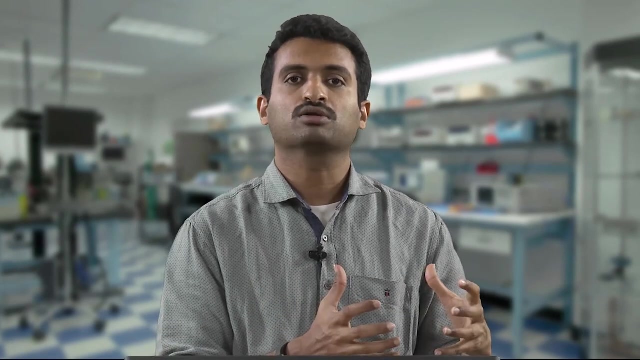 and that is what we see here, And obviously the inverse of it. when Pe is greater or greater than your particular reference, what does that mean? low activities of your particular electron and that would correspond to lower concentrations of your particular reduced species or higher concentrations of your oxidized species, meaning oxidizing conditions predominate. 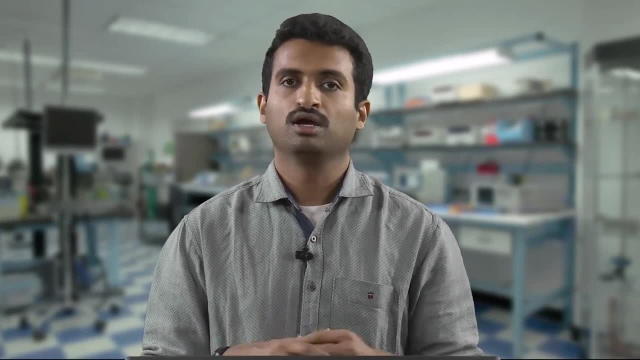 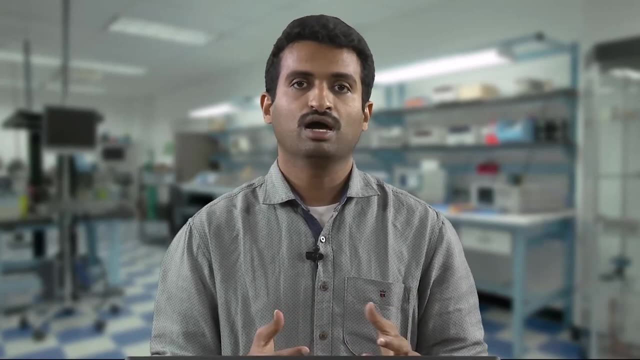 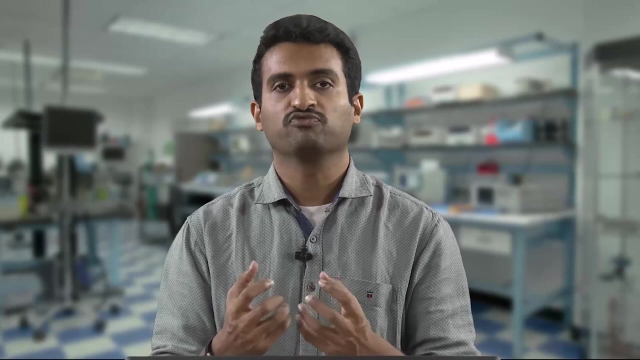 So thus a oxidized form would predominate, and how can you understand this? it is similar to our pH and pKa graph That you looked at, and similarly, a reduced form would correspond to the acid, which is the compound with the proton, and a oxidized form, meaning the compound without the electron. 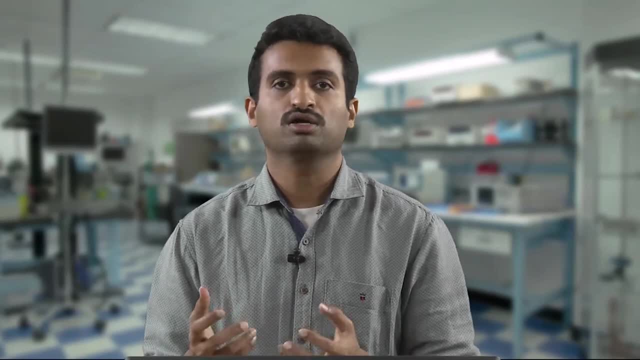 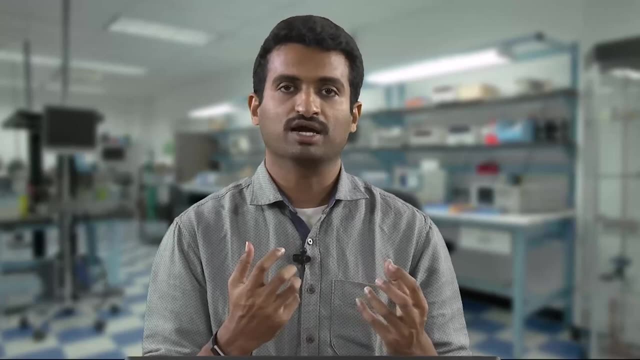 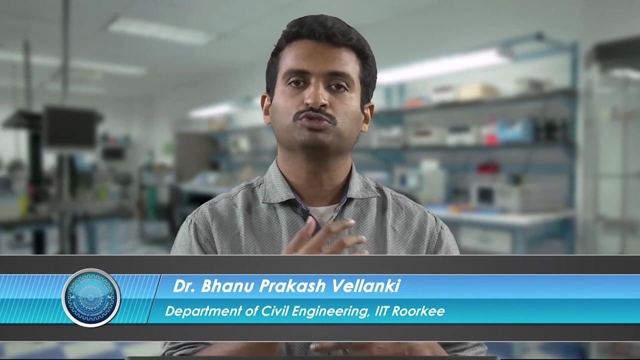 would be similar to the compound without the proton or A-. With that I will end today's session, and we are now going to look at how can I look at two half reactions and the relevant Pe1 or Pe values or the reduction potential values, and then be able to understand which particular compound will then act as the oxidizing agent.